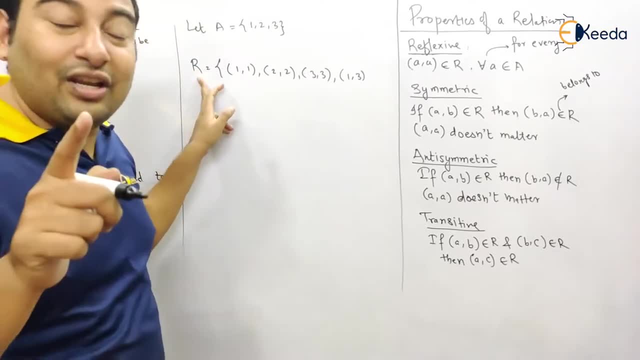 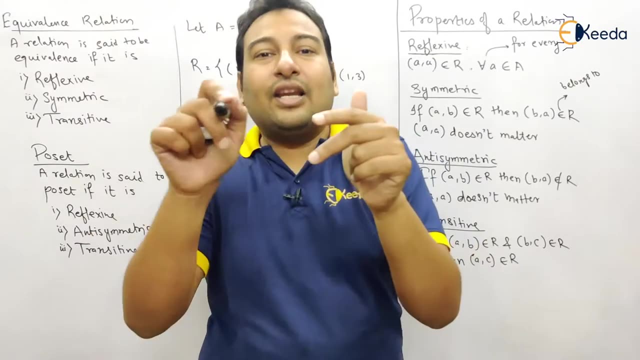 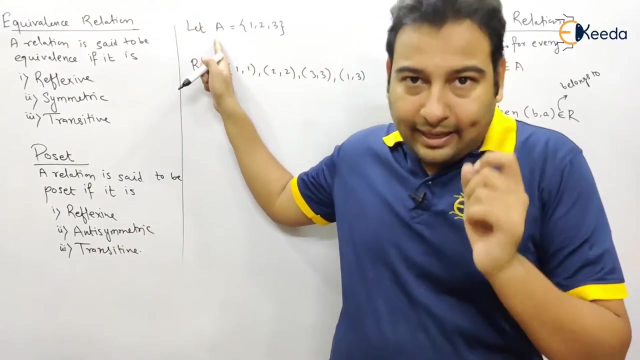 way of writing down a relation r. So please tell me, this relation is from where to where? From a to a, If there are two sets, a and b, and a relation is defined, so we can say it's a relation from a to b if it is a subset of a cross b. But here, in this case, there is only one set, a, and a relation is. 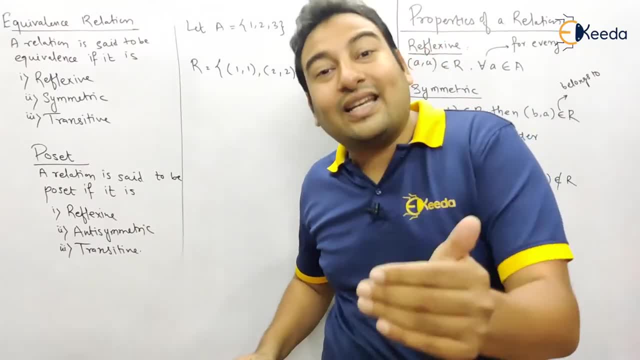 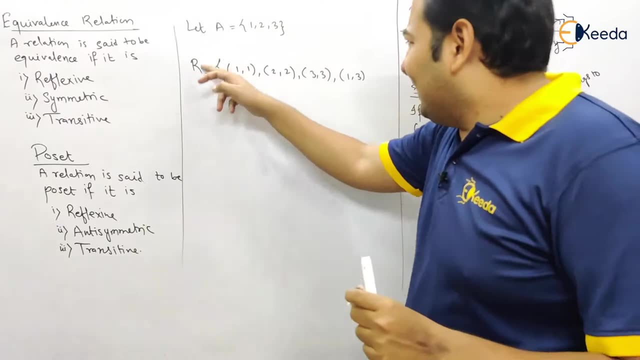 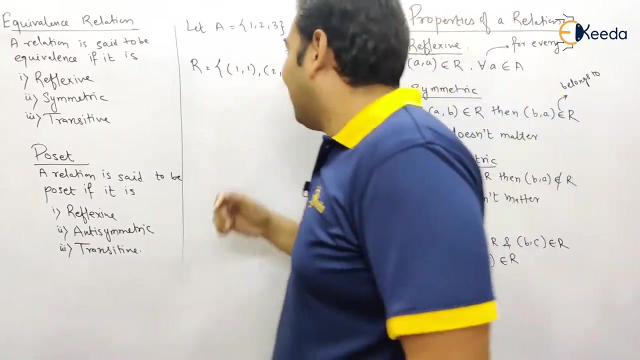 defined. so obviously it's a relation from a to a and it has to be a subset of a cross a. So this is not the point of discussion here. Whatever I'm writing here in r is by default. it's a subset of a cross a. Therefore it's a relation from a to a. So let 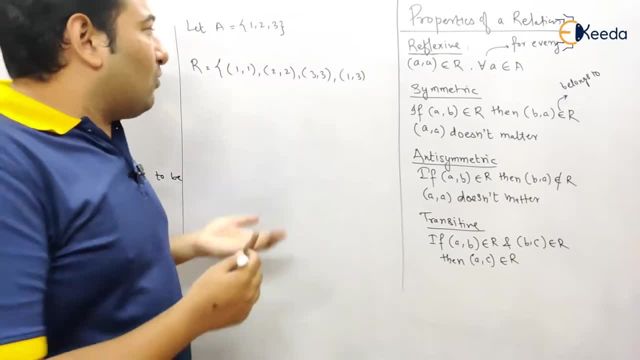 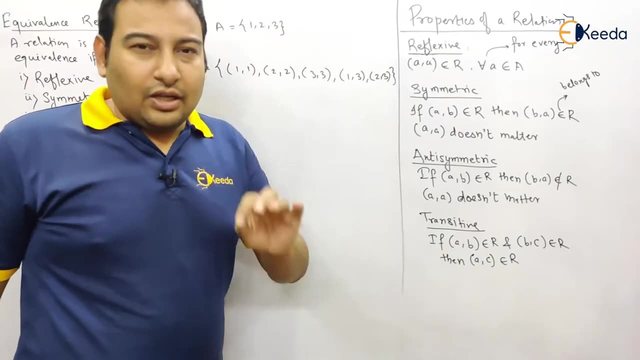 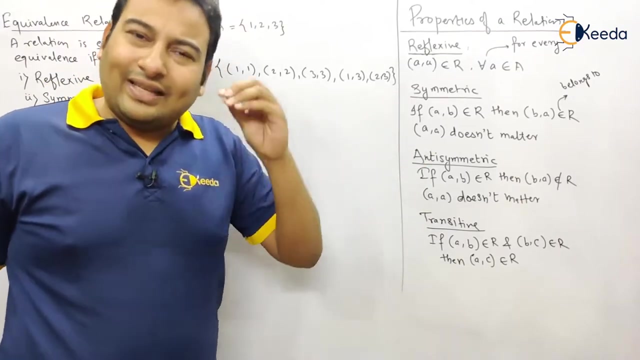 us start. So see here: if it is a subset of a cross a, then two comma threes may be present. so there is no problem. Is it reflex you? Yes, So what reflex you says? all this self element must be present. Other elements doesn't matter. whether they are present or does not present, It doesn't matter. 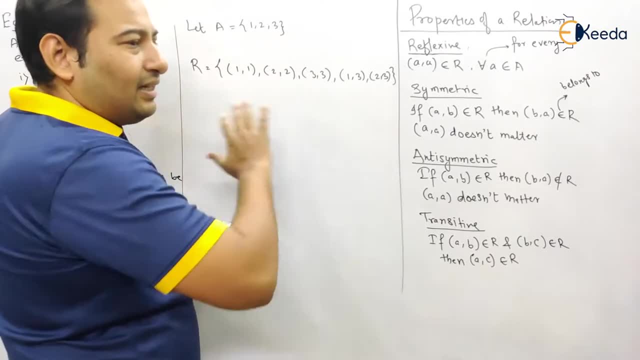 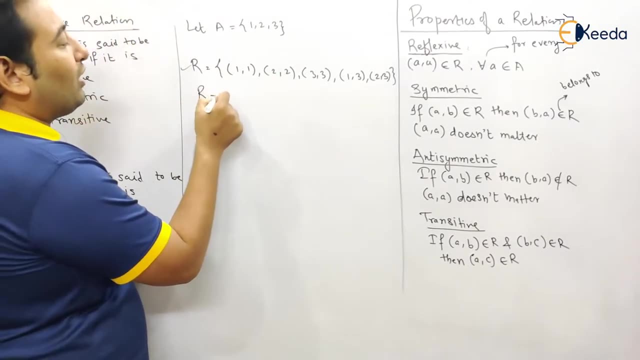 to us, See here. So if there is one, one, two, two, three, three, that's it. It's a reflex you. If these elements are there or not there, doesn't matter to us, It's reflex you, What about? So? it's a reflex you. What about this? 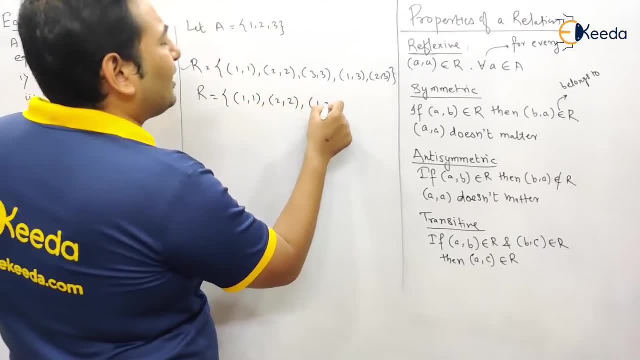 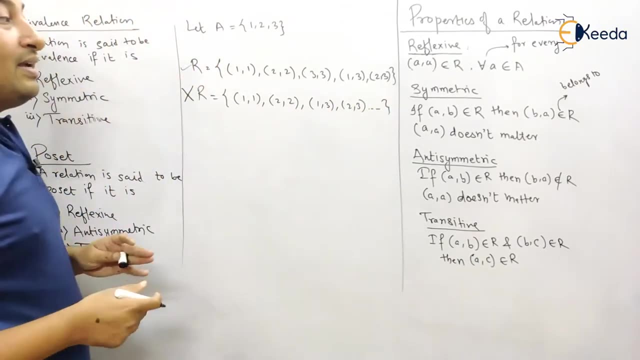 Suppose there is one one, Suppose there is two, two and lot of other elements. Let's say one, three, two, three and lot of other elements. Obviously all belongs to a cross a. Is it reflex you? No, Why? Because the reflex you criteria says all the self element must be present. So one one is there two. 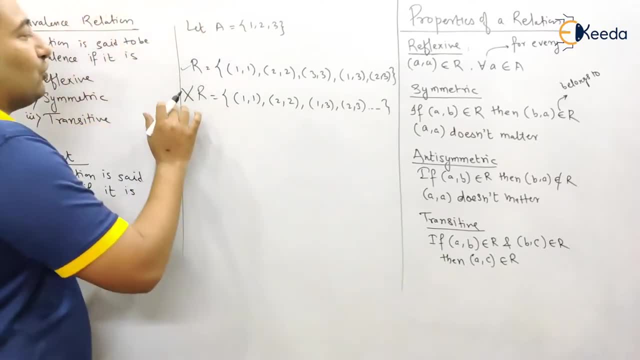 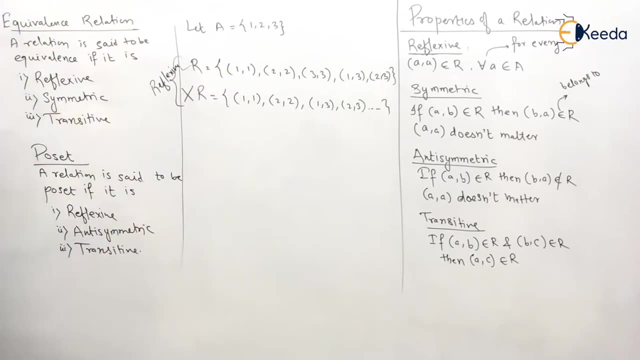 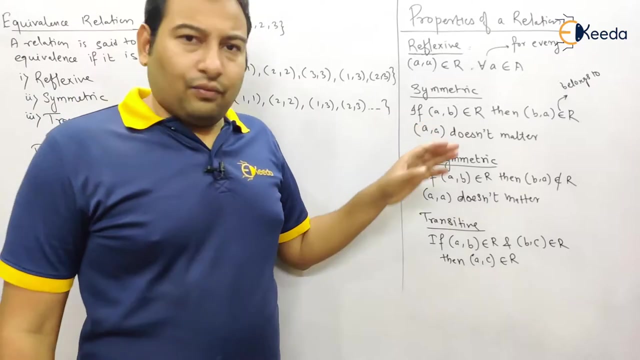 two is there, but three, three is not there. So if there is one, one, two, two, three, that's it. It's a reflex you. I hope the reflex you definition is clear. So the first set is a reflex you. Second set is not the reflex you. Now let us discuss the next property: symmetric. Very simple definition. 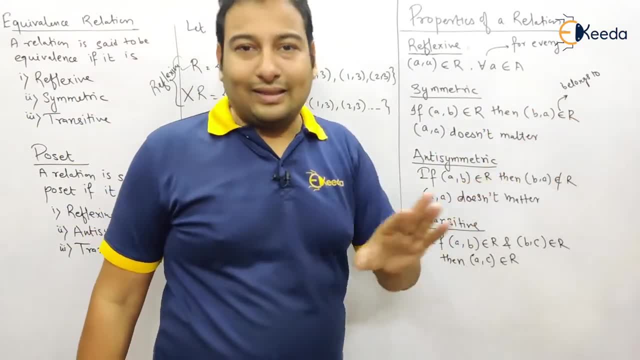 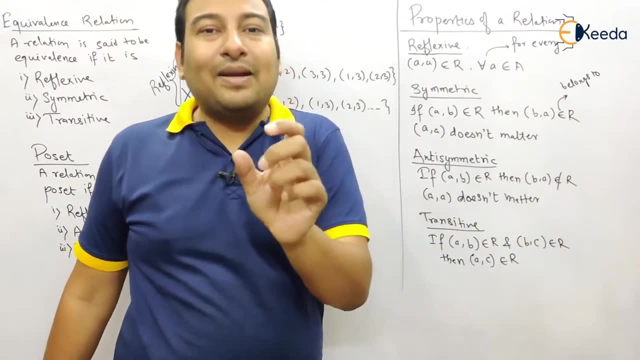 again: If a comma b belongs to r, then b comma belongs to r. that's it. If a comma b belongs to r, then b comma belongs to r. A comma a doesn't matter. The self element here doesn't matter whether they are present or not present. So a comma b belongs to r, then b comma i belongs to r. 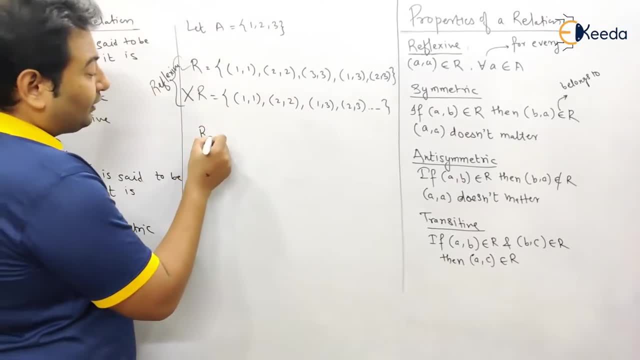 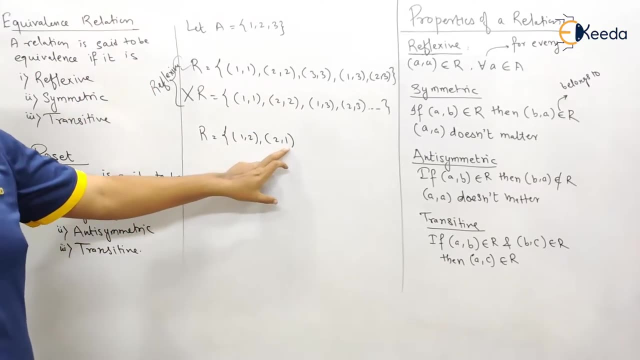 present doesn't matter. for example, let me write it on a relation: let's say 1 comma 2 and let's say 2 comma 1. see here: a comma b, b comma a, a comma b, b comma a, reverse. if only this is the relation. 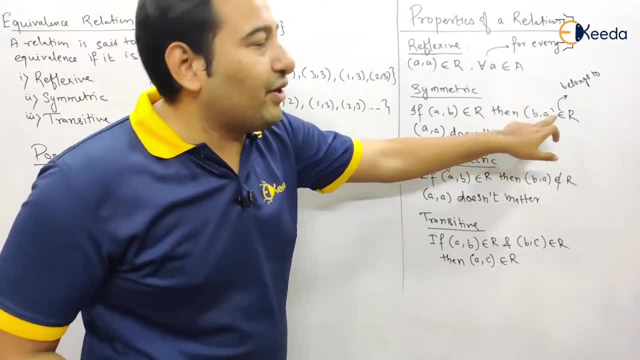 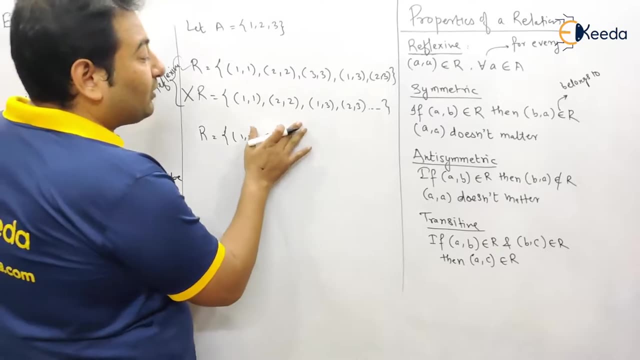 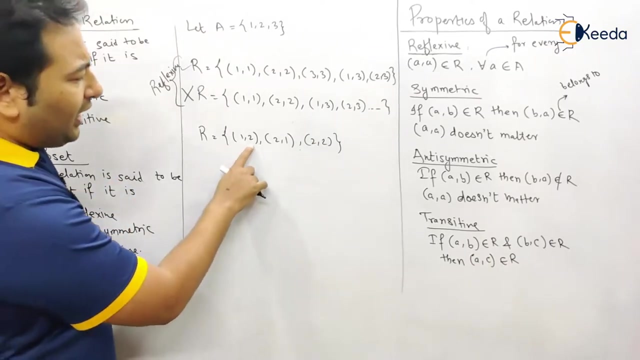 then it is a symmetric. why? because a comma b, b comma a. that's a story over 1 comma, 2 and 2 comma. both are present. it's a symmetric relation. what about this if i'll add 2 comma to this, to this relation? so what will happen? see, it's very simple. a comma, b, b comma, a self element, doesn't matter. 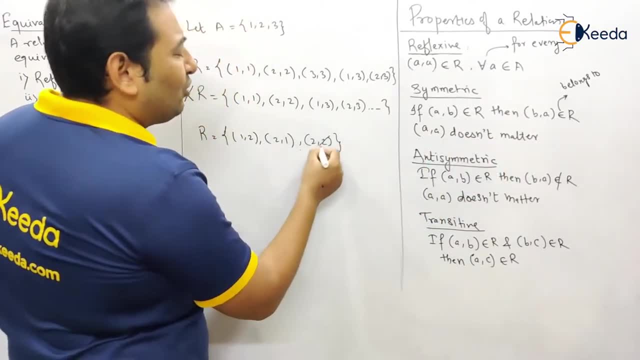 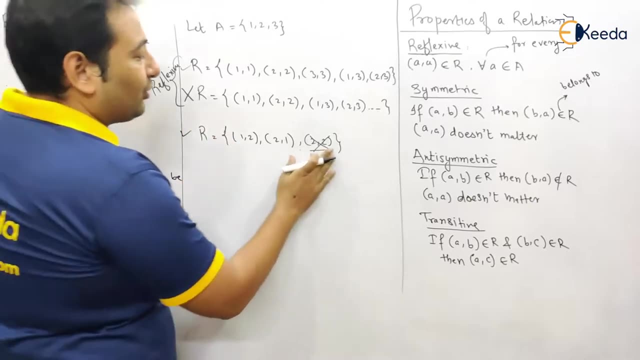 a comma doesn't matter, so actually this doesn't matter to us, so the conclusion will be based on this: a comma b, b comma a. therefore it's a symmetric relation. are you clear with this? let me write it on one more relation to check whether you understood or not. 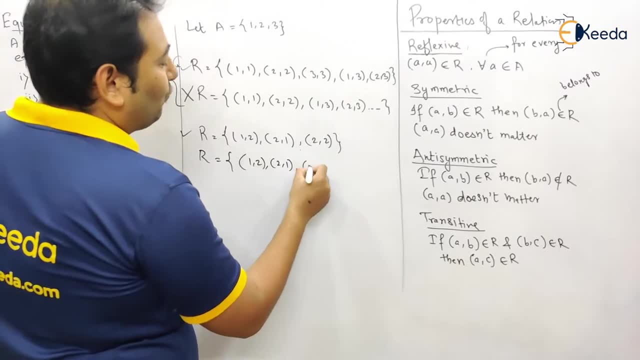 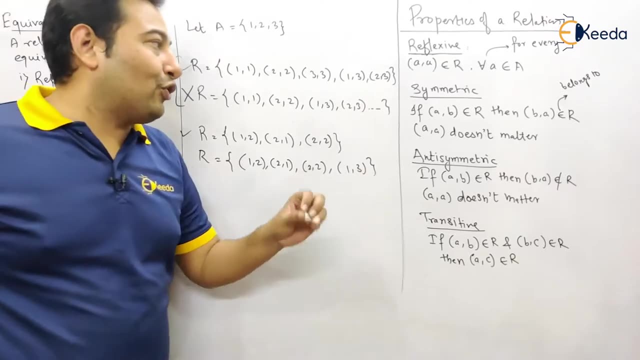 you. let's say you have 1 comma 2. let's say you have 2 comma 1. let's say you have 2 comma 2. let's say you have 1 comma 3. please tell me whether this relation is a symmetric relation or not. 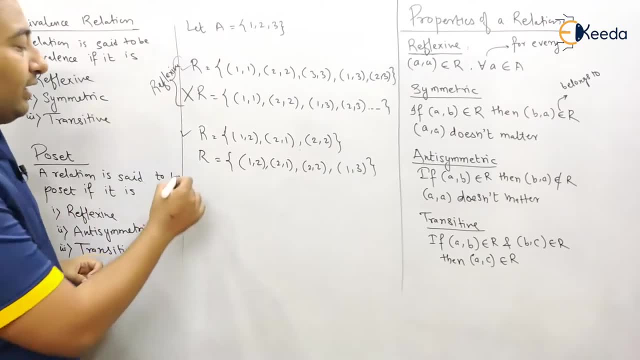 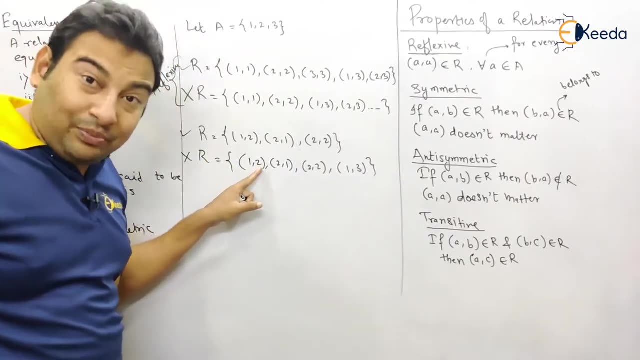 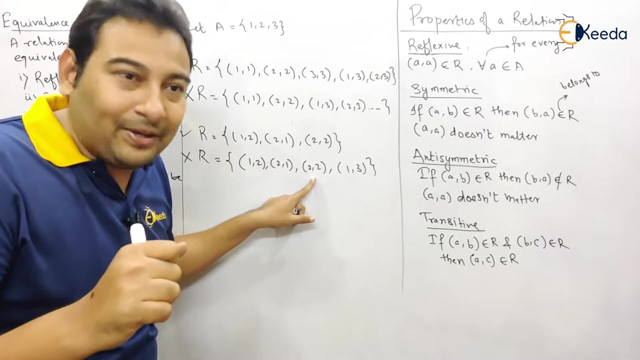 it's not a symmetric relation. why? because see a comma b, b comma a satisfying the criteria. if a comma b is present, b comma a must be there, so it's a satisfying criteria. this term doesn't matter to us because we are not bothered about the self elements. what about this? 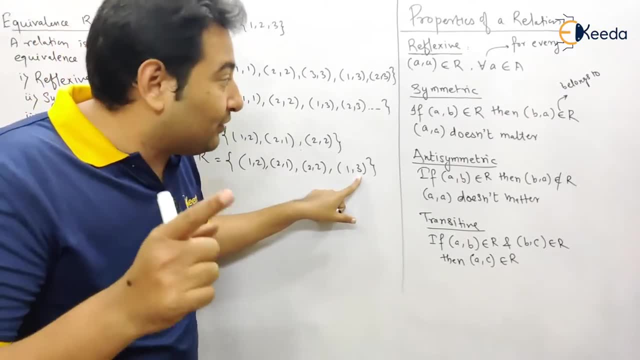 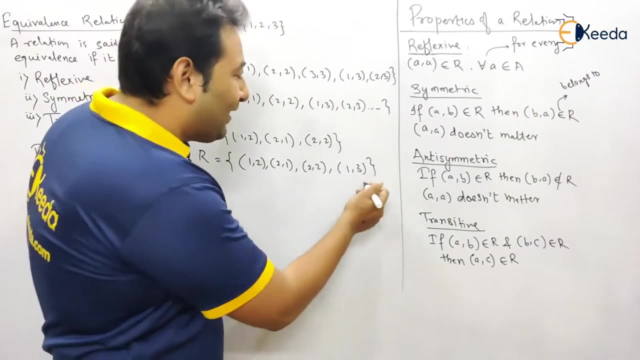 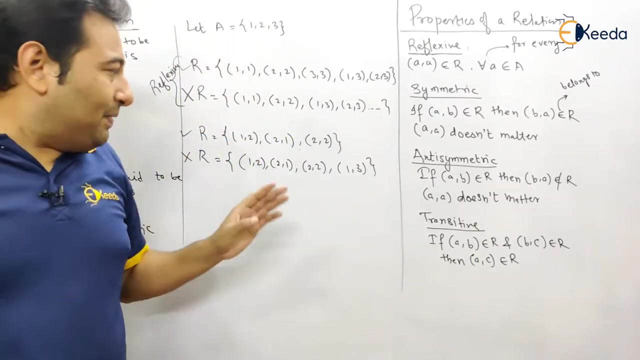 1 comma 3 is present, then 3 comma 1 must be there. see here: if a comma b is present, b comma a must also be there. therefore this term is not satisfying the criteria. therefore the whole relation is not a symmetric. there may be n possibilities which are satisfying the criteria, n pairs satisfying. 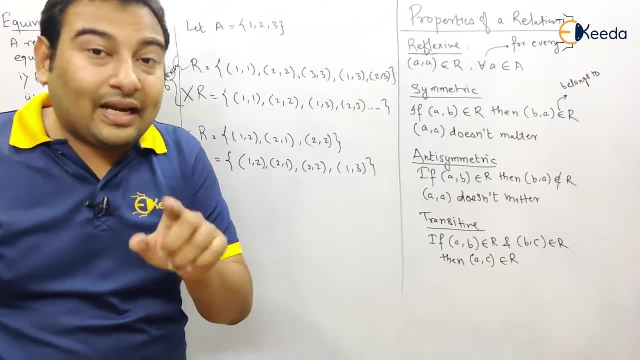 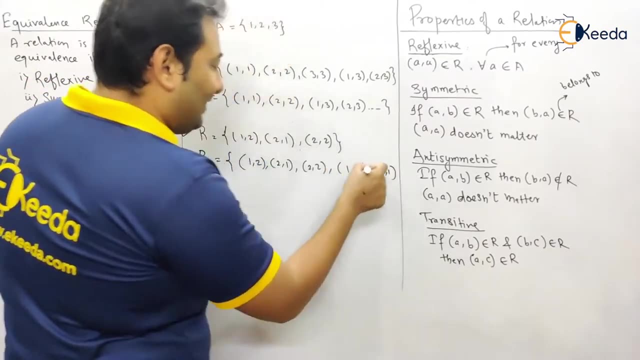 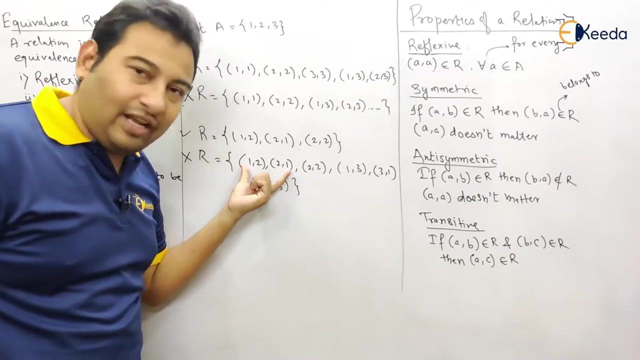 the criteria. if only one pair not satisfying the criteria, it's not symmetric. so suppose let's say you have 3 comma 1, again, this is satisfying. then you have 2 comma 3, again it's not a symmetric relation. this is satisfying. a comma b, b comma, this is also. 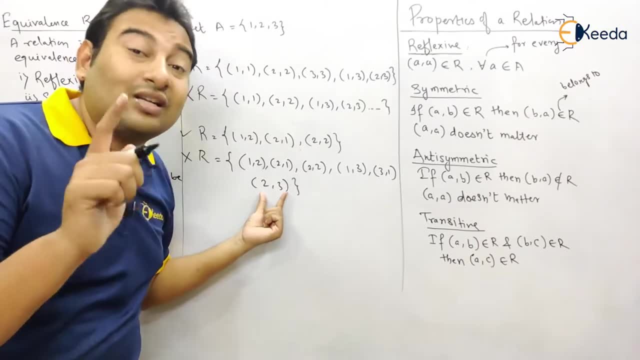 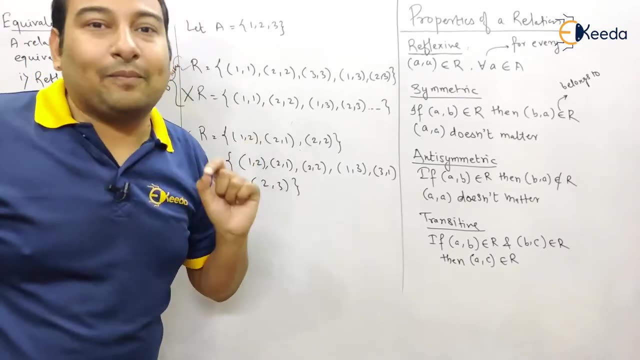 satisfying. this doesn't matter to us. there is only one pair which is not satisfying the criteria, because 2 comma 3 is present. if it is present in a relation, then 3 comma 2 must be there. there is only one pair which is not satisfying the criteria. that means the entire relation is not symmetric. i. 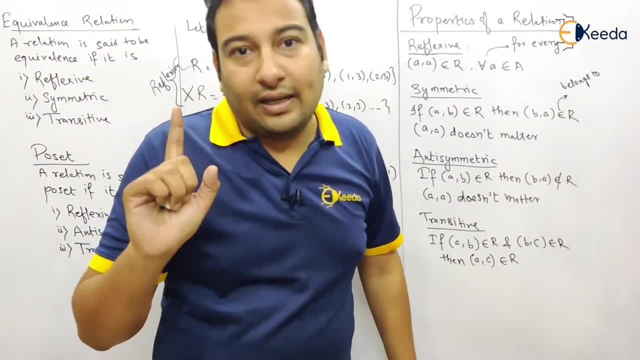 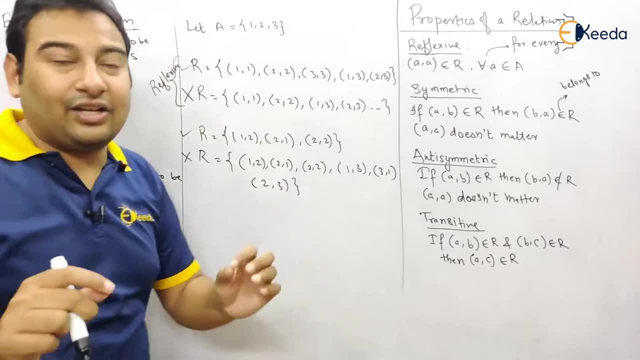 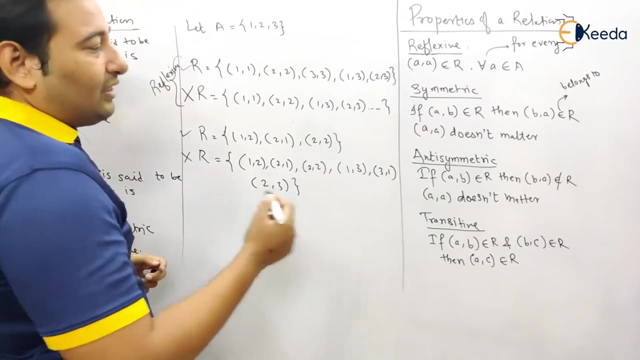 hope this is clear. all the pairs must satisfy the criteria. if there is, if there are, let's say, 99 pairs which are satisfying, only one pair is not satisfying, then the relation is not symmetric. is this clear? so this is the discussion about symmetry. next let us talk about anti-symmetric. 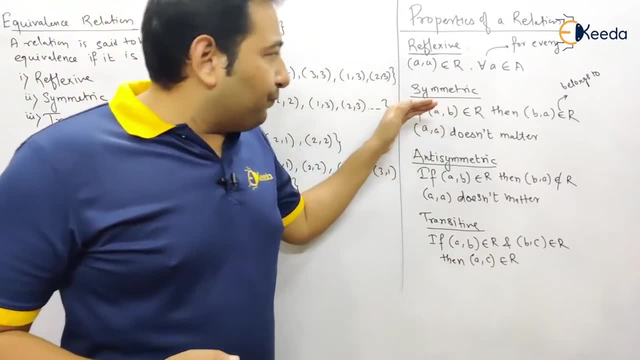 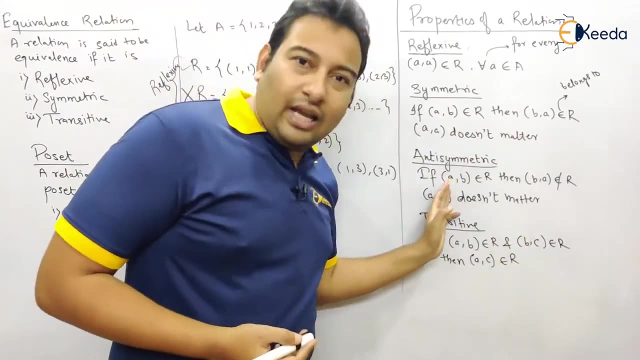 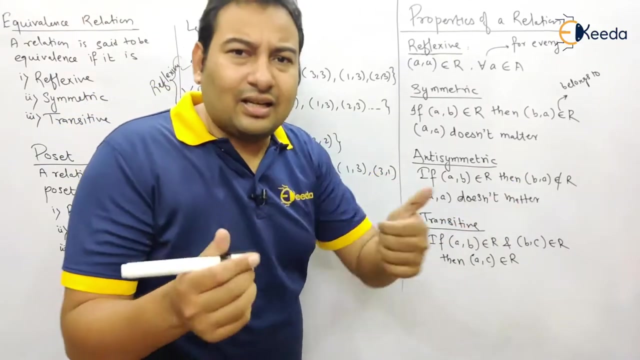 very simple opposite to symmetric. what is symmetric saying: if a comma b present, b comma must be there. here a comma b. if it is present b comma must not be there. so exactly opposite. if a comma b is there, b comma a does not exist, that's it. and here also the self element doesn't matter. for example, suppose if i'll 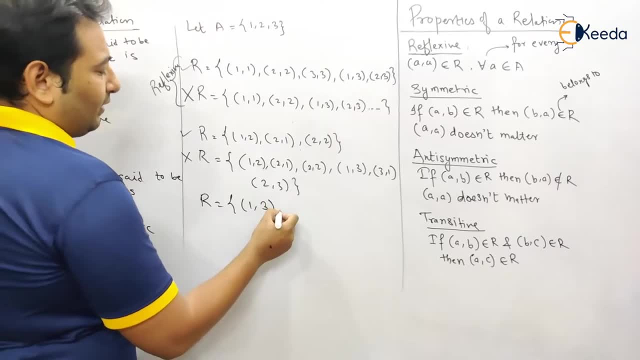 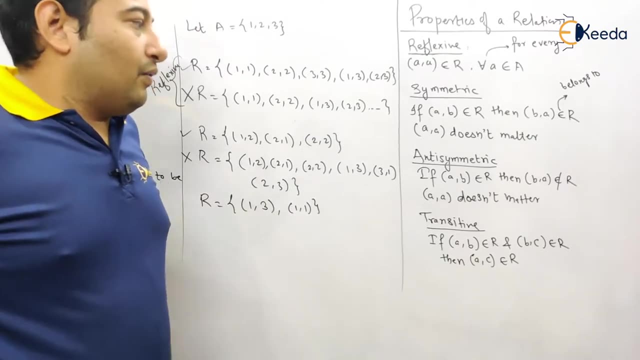 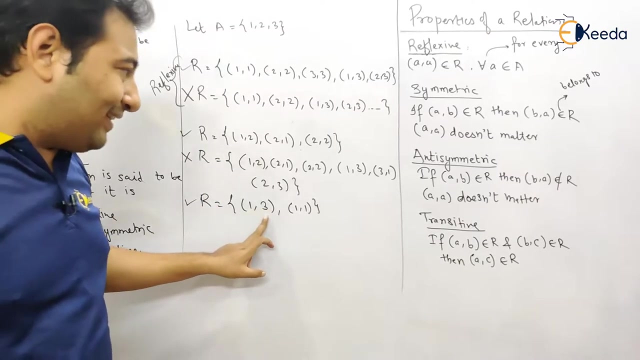 say 1 comma 3, let's say 1 comma 1. please tell me whether it is an anti-symmetric relation or not. whether it is an anti-symmetric relation or not, yes, it's an anti-symmetric relation. why? because, see here, 1 comma 3 is there and 3 comma 1 is not present. means a comma b is present but b comma is not there. 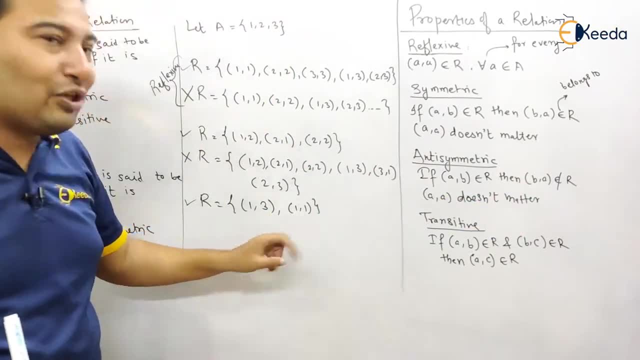 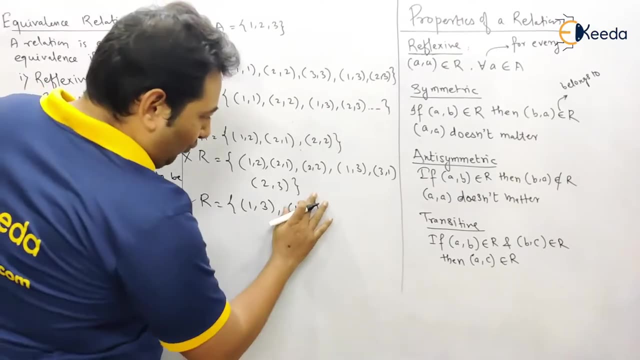 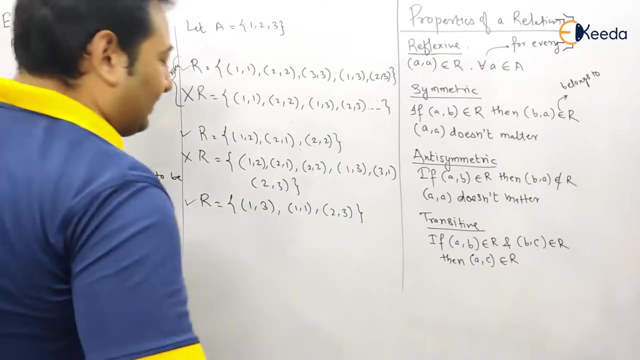 so 1 comma 3 is there, 3 comma 1 is not there, and this term doesn't matter to us. therefore it's anti-symmetric. are you clear with this? suppose? what about this term? is it anti-symmetric? yes, again, it's anti-symmetric, because 1 comma 3 present 3 comma 1, not present. 2 comma 3 present 3 comma 2. 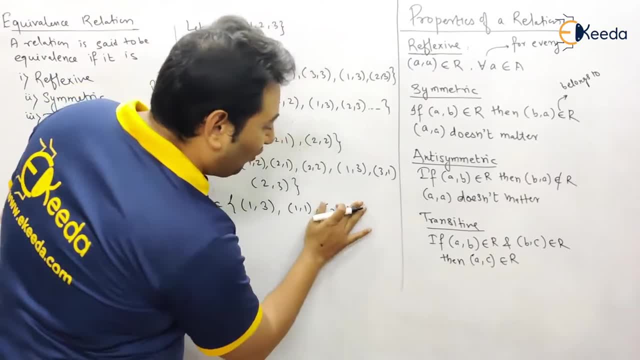 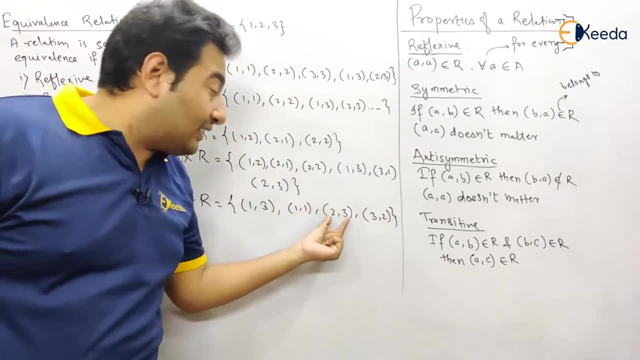 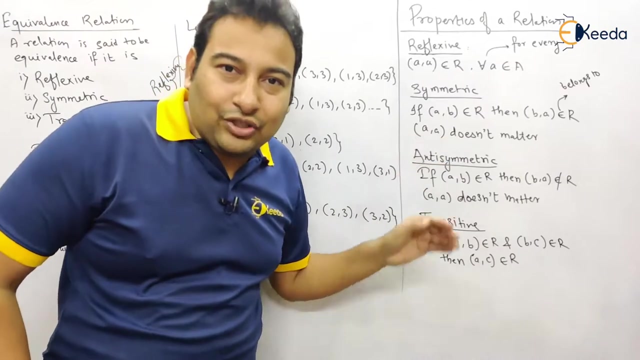 not present. self-element doesn't matter to us. what about this? now? in this case it is not anti-symmetric. why? because a comma, b and b comma. both are present. again the same point, the point that we discuss for symmetric. the same is valid for anti-symmetric. 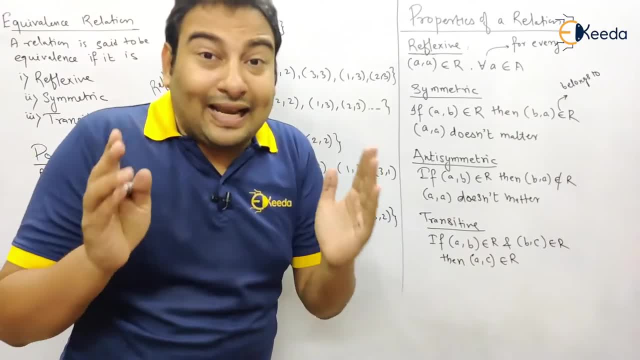 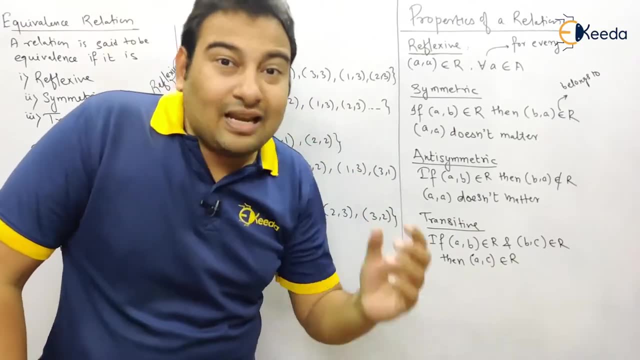 and the point is there. the point is that if there are 99 pairs satisfying the criteria, only one pair not satisfying the criteria. that means there are anti-symmetric and there are anti-symmetric pairs. number of pairs satisfying the criteria: only one pair not satisfying the criteria: the whole. 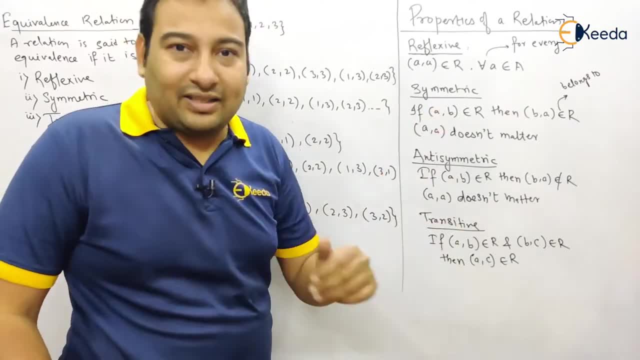 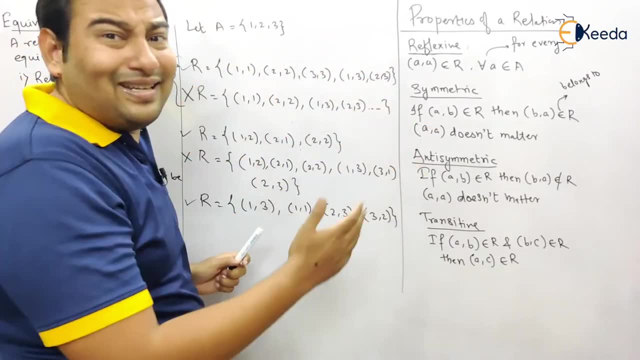 relation will be not will be symmetric, not will be anti-symmetric. what i'm saying, see here, because of this term, it is anti-symmetric. because of this term it is anti-symmetric. and let's say there are number of term. because of that it is anti-symmetric. suppose there is one more term. 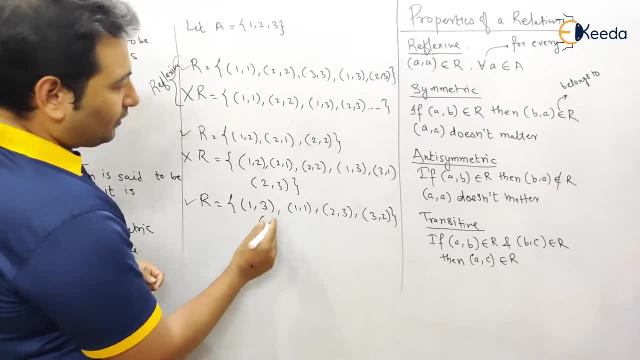 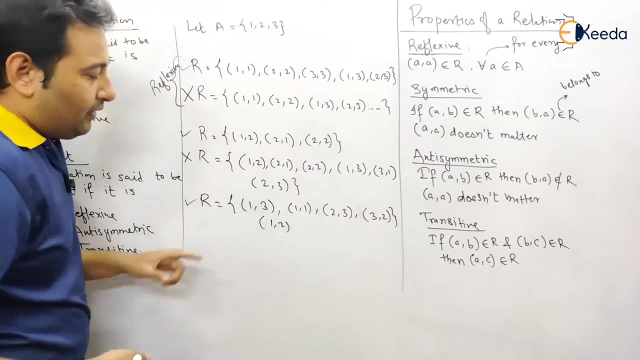 let's say 2 comma 3 is done. let's say 1 comma 3. let's say, uh, 1 comma 2, see: anti-symmetric because 3 comma 1 is not present. anti-symmetric because 2 comma 1 is not present. it doesn't matter to us. 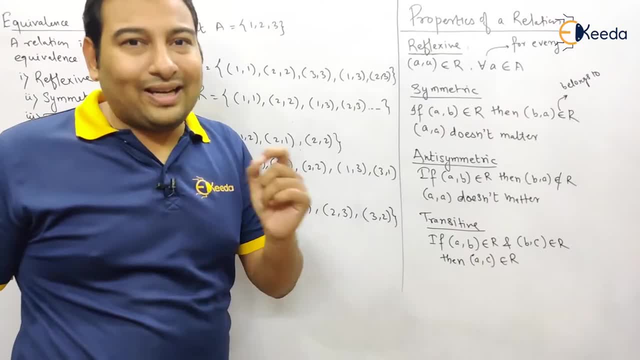 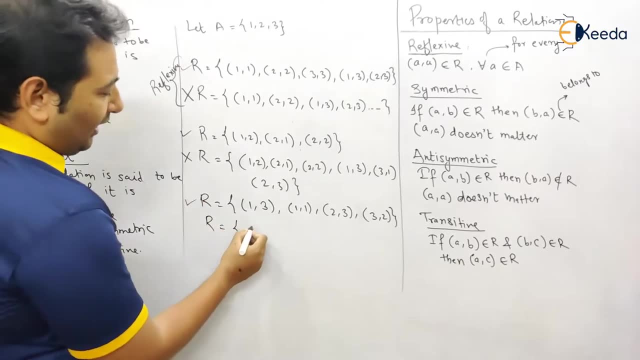 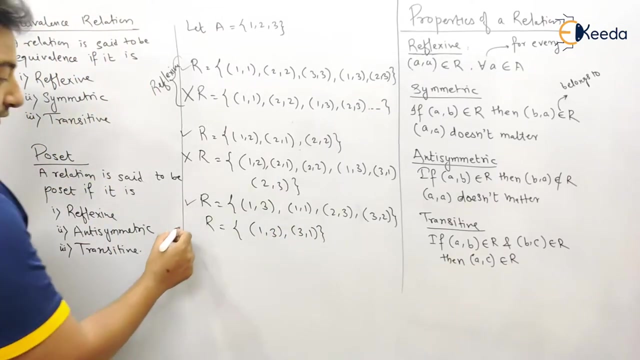 but this term is not satisfying the criteria. therefore, the whole relation is not a anti-symmetric. i hope this is clear. this is symmetric. and suppose- sorry, this is anti-symmetric- and suppose if i write something like this, then it is not anti-symmetric. so this is your example for symmetric. basically, 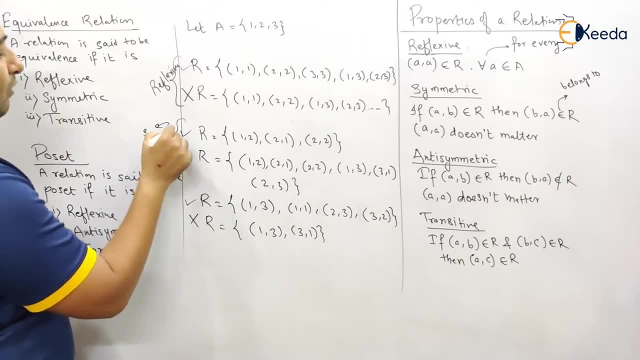 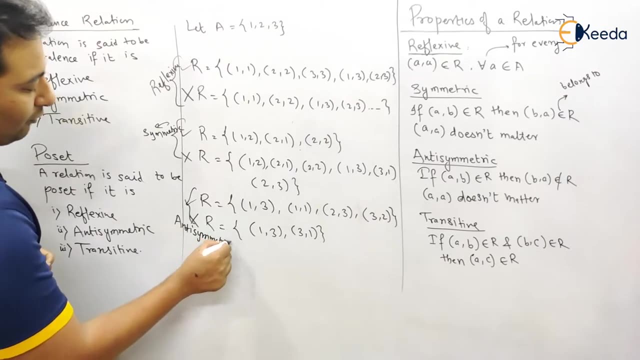 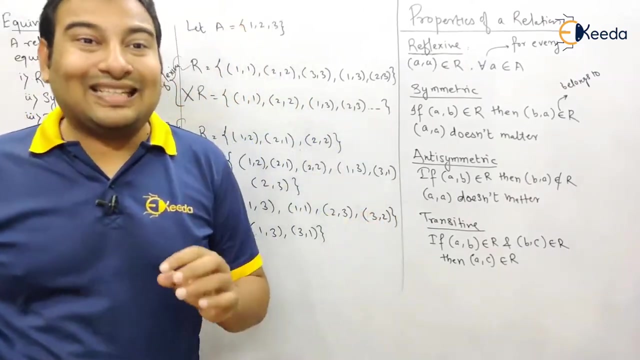 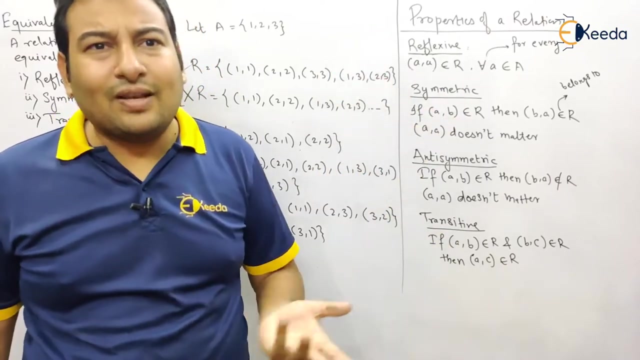 and this is your example for symmetric. basically, this is the discussion for anti-symmetric. now you might be thinking. a question may come in your mind and see, this is a very popular topic that comes in gate exam as well, as you can think of your mcq paper. if you have mcq paper, this is a very popular question. 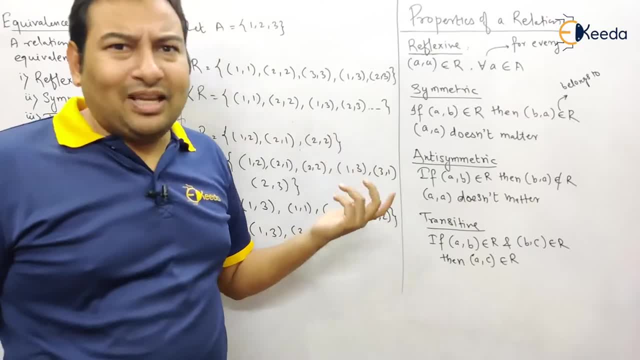 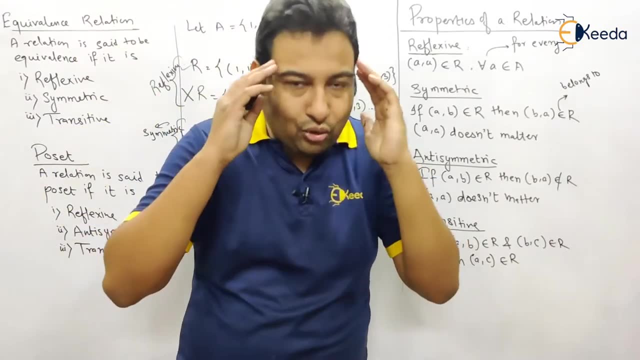 properties of a relation. a relation may be given and it is. it will be asked whether it is symmetric, anti-symmetric, or what are the different criterias, and so on. so this is very important topic, so you should be very clear with the topic now. the question is: is there any relation which is 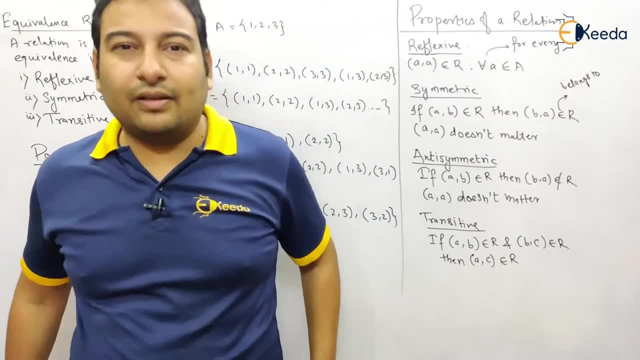 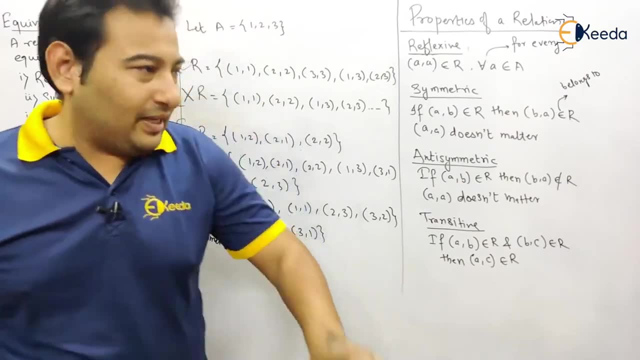 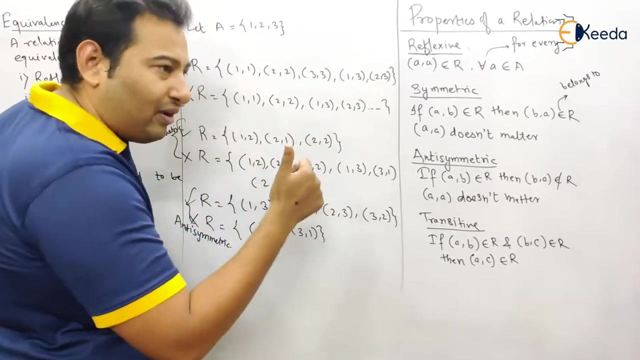 symmetric as well as anti-symmetric? please tell me this. the question is for you: is there any relation which is symmetric as well as anti-symmetric? because see here, see here, this relation is symmetric, this relation is symmetric, but it is not anti-symmetric. why see self element doesn't? 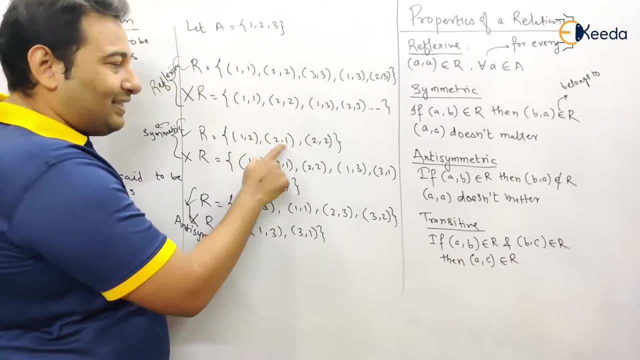 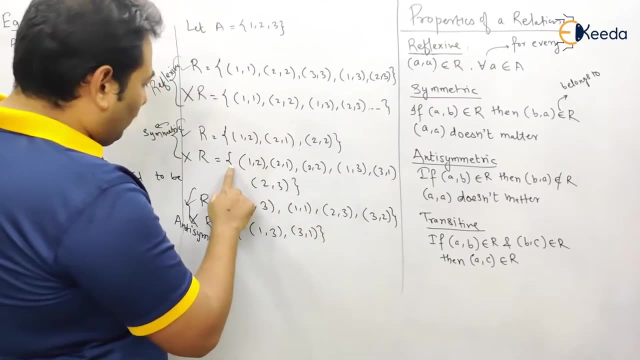 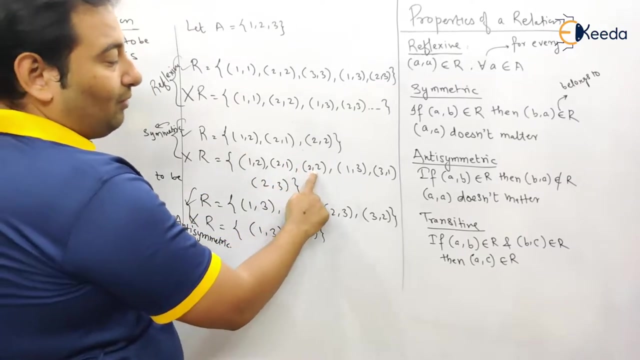 matter. a comma b is present. b comma s present. that means it is symmetric. since it is symmetric is symmetric, it is not anti-symmetric. what about this? this is also symmetric. no, it's not a symmetric because of this term. 1 comma 2, 2 comma 1. 2 comma 2. 1 comma 3, 3 comma 1. 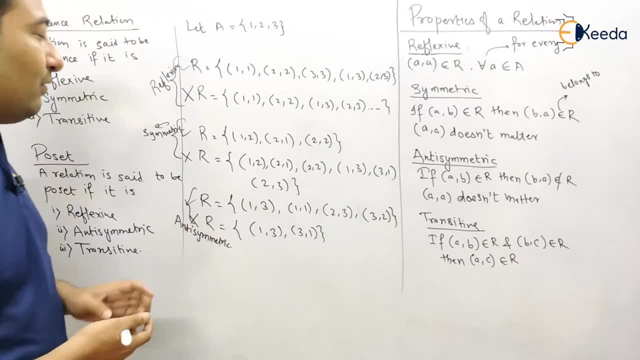 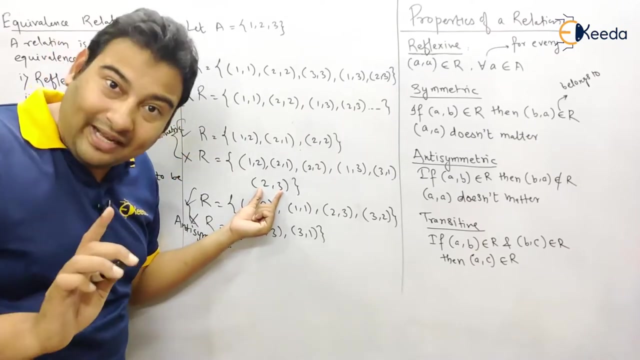 2 comma 3. what about is? it is not a symmetric. please tell me, is it anti-symmetric? so this relation is not symmetric as well as not anti-symmetric. why it is not symmetric? because 2 comma 3 is present, but 3 comma 2 is not present. therefore it is not symmetric. 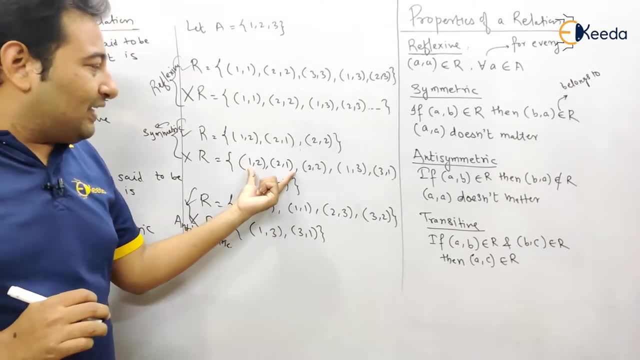 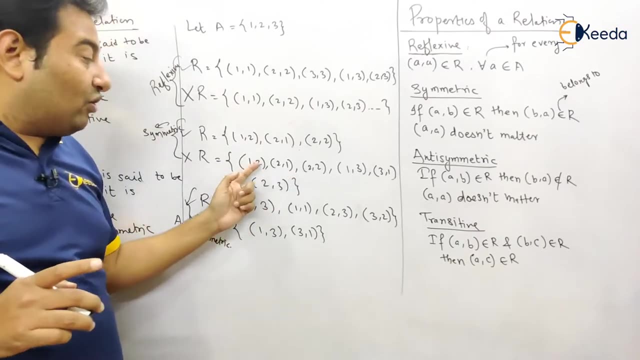 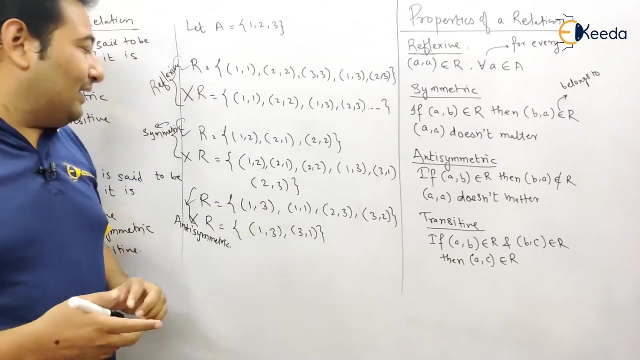 what about anti-symmetric? see, because of this criteria, it is not anti-symmetric, because what the criteria of anti-symmetric says: 1 comma 2 is present. 2 comma 1 is also present. a comma b present, b comma must not be present. therefore, this particular relation is neither. 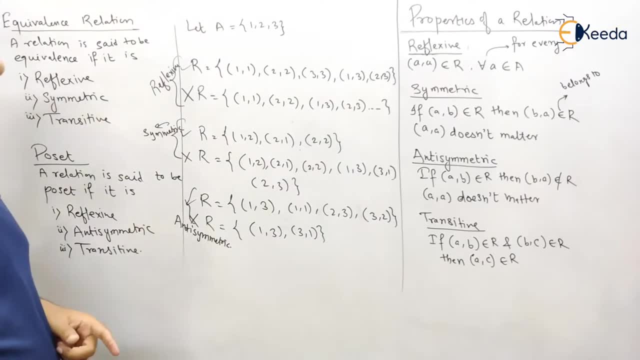 symmetric not nor anti-symmetric. is this clear? my point is: i am looking out for a relation which is both symmetric as well as anti-symmetric. what about this? this is symmetric, not anti-symmetric. this is neither symmetric nor anti-symmetric. what about this? this is neither symmetric nor anti-symmetric. why? 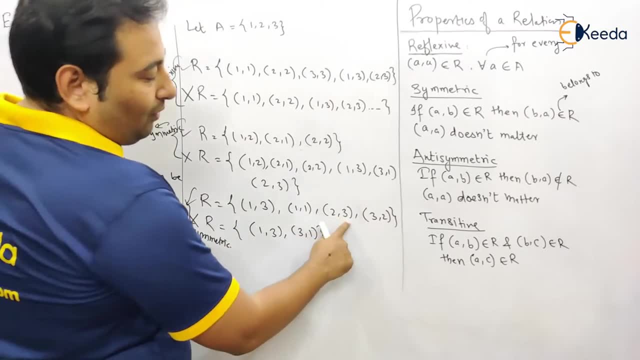 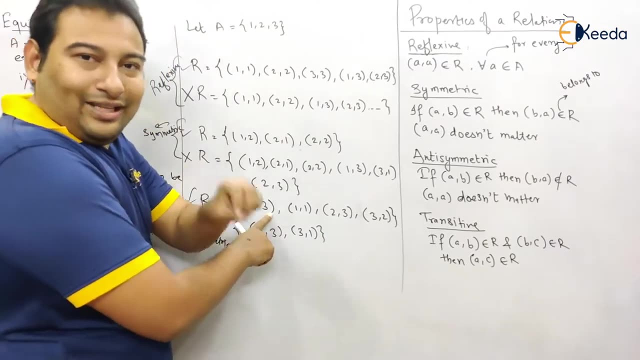 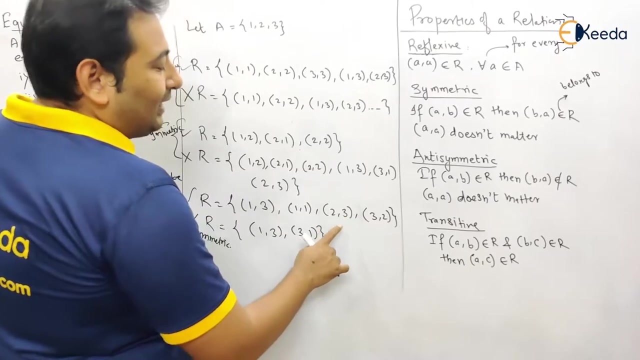 see here, because 1 comma 3, see 2 comma 3, 3 comma 2. that means symmetric criteria satisfied, but 1 comma 3, but 3 comma 1 is not present. therefore it is not symmetric. and what about anti-symmetric? again, it's not anti-symmetric because a comma b, b comma, i, both 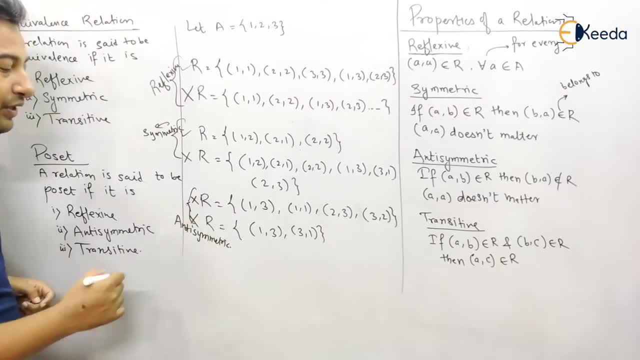 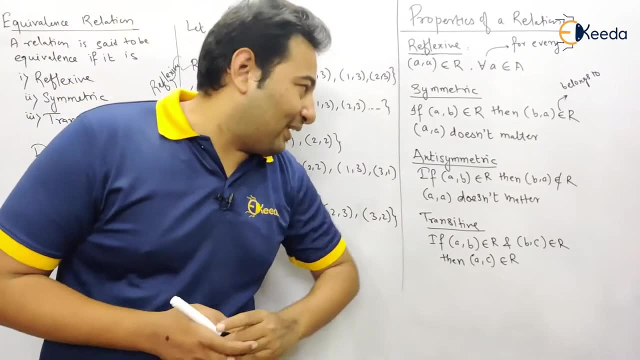 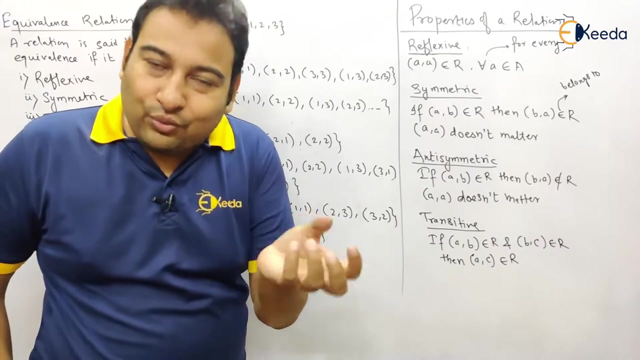 are present. therefore, it is neither symmetric nor anti-symmetric. and what about last? it's symmetric but not anti-symmetric. so this is the discussion on symmetric and anti-symmetric. now my point is: you have seen the different cases in which there were few relations which were symmetric. 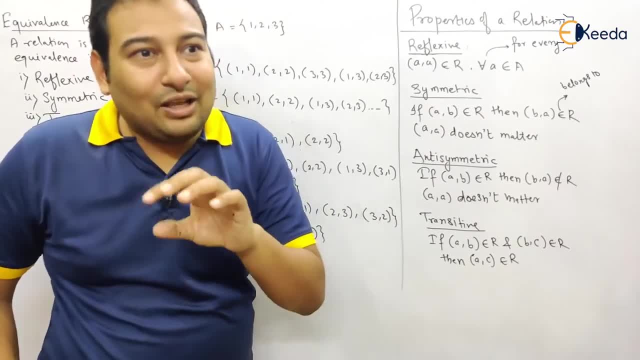 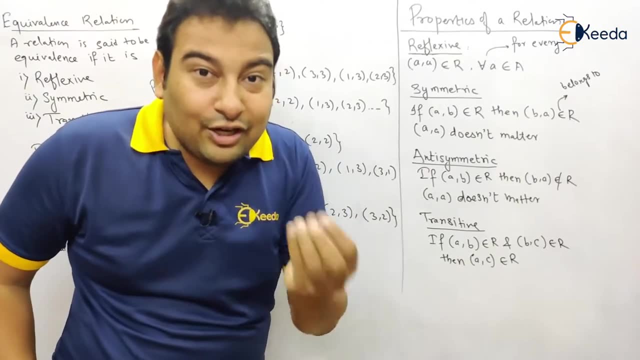 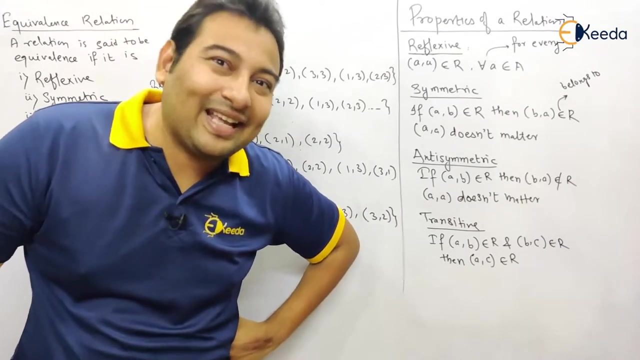 there were few relations which were anti-symmetric. there were few relations which were neither symmetric nor anti-symmetric. my point is: i'm trying to ask you one question: can you tell me a relation which is symmetric as well as anti-symmetric? please tell me. can you tell me a relation which is symmetric as well as anti-symmetric? 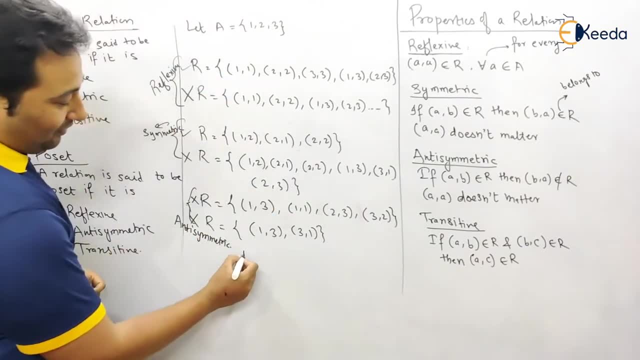 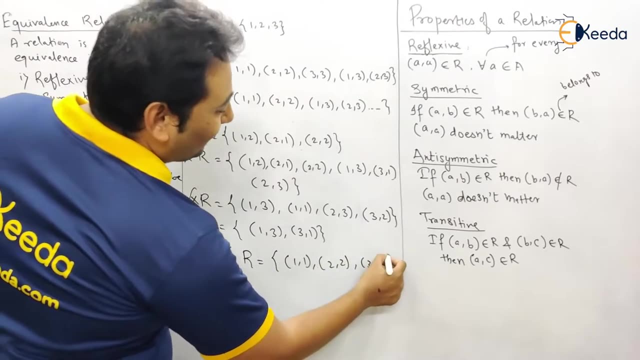 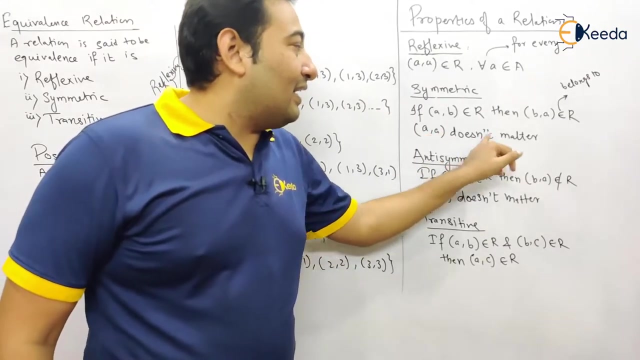 yes, there is a relation, and the relation is: suppose you have 1, 1, 2, 2, 3, 3. please tell me now what about this relation? see, in symmetric as well as anti-symmetric, in anti-symmetric doesn't matter to us. so it doesn't matter to us, that's it. so if this is a 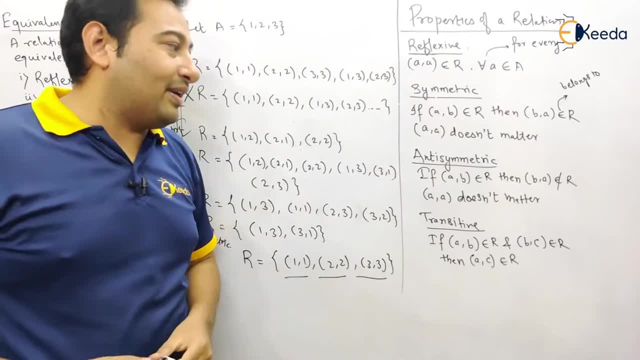 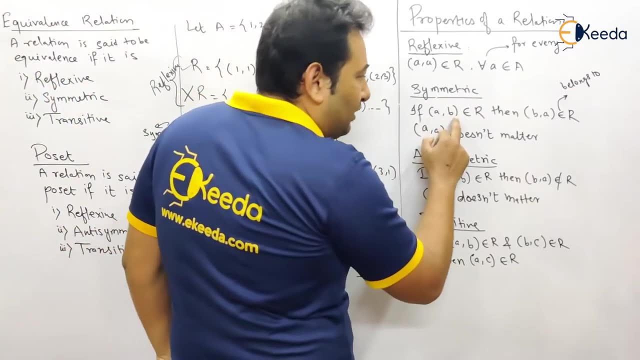 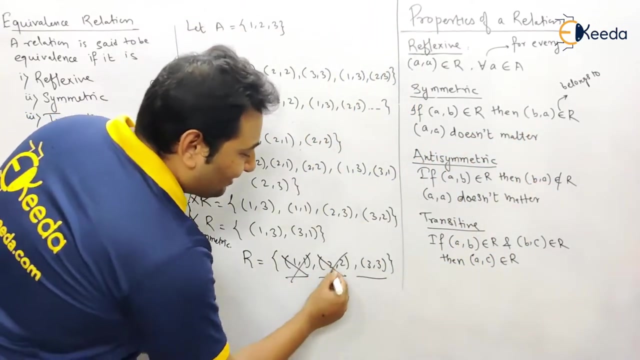 relation, then it is symmetric as well as anti-symmetric, because, see, the criteria is very simple. what is the basic criteria? if, then, statement means: if this is present, it has to present. if this is present, this has to be present and this doesn't matter to us. so this doesn't matter to us. this. 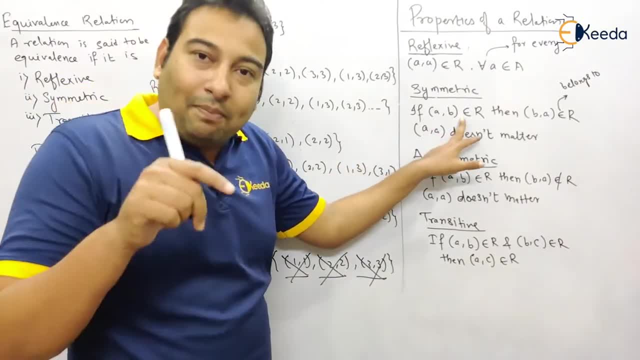 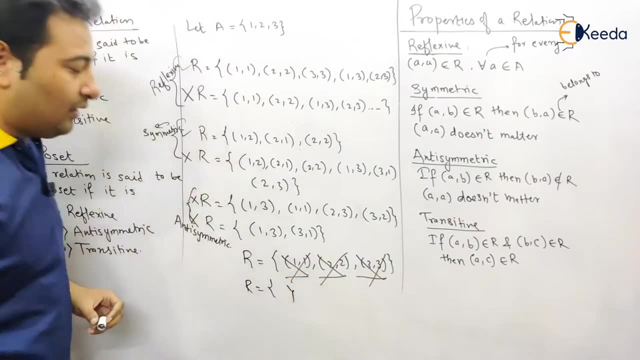 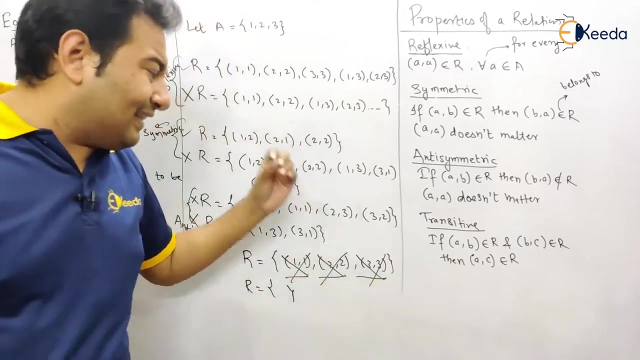 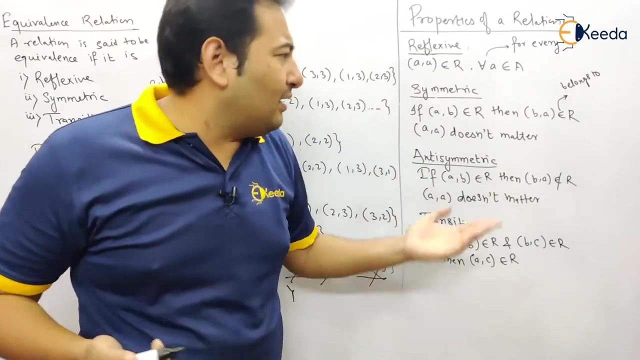 doesn't matter to us. this doesn't matter to us. if a comma b present, then b comma a must be there. if it doesn't matter to us what we are left with, we are left with nothing. basically what we are left with. we are left with basically nothing. because this doesn't matter to us, that means in a resultant relation, a comma b is not present. if a comma b is not present, we are not bothered whether b comma is there or not. 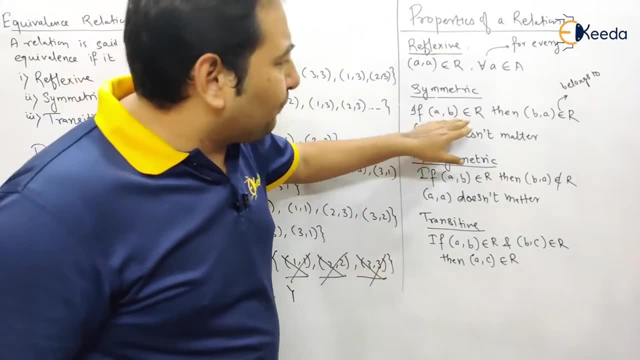 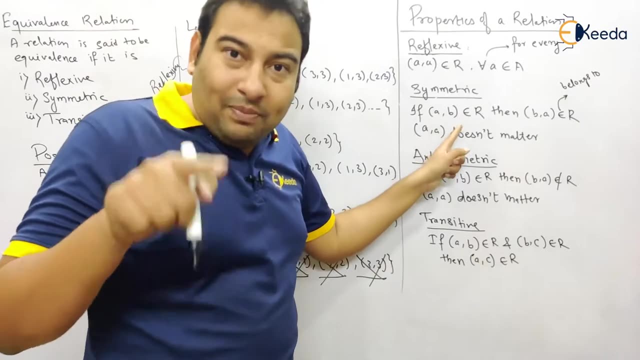 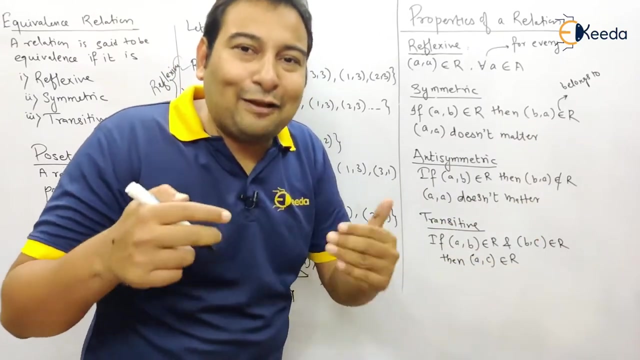 see when to check. if a comma b is present, then we going to check whether b comma is present or not. if a comma b is present and b comma a present, then is symmetric. if a comma b present and b comma i not present, it is anti-symmetric. but if there is no a comma b, then what? 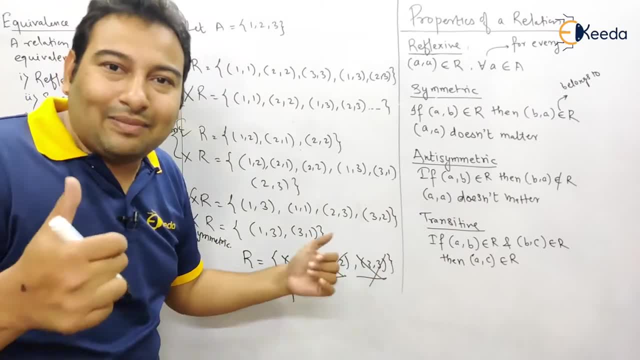 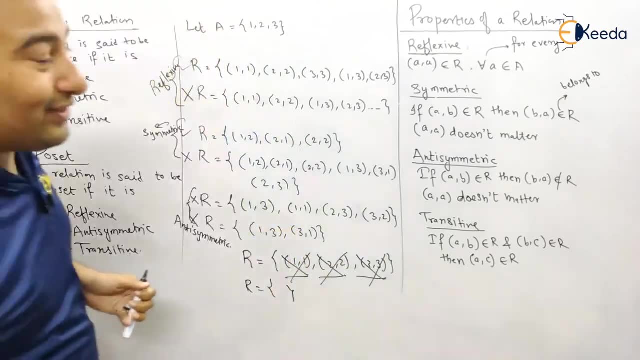 see here there is no a comma b because only self element. that doesn't matter to us, so there is. if there is no a comma b, then a relation is symmetric as well as anti-symmetric. is this clear? am i made my point clear or not see? this may be confusing for you. 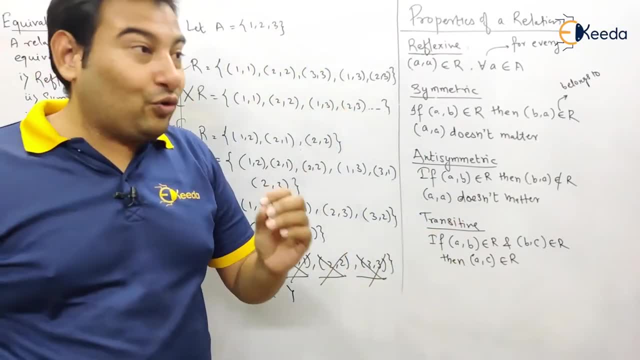 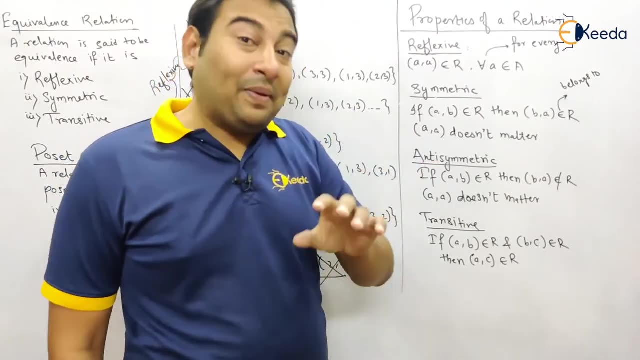 but you don't have option. this video is very important. you need to watch this video two times, three times, four times, till you understand, because the next topics- few topics- will be based on this and very likely you can get- uh, you're going to get- the problems based on this in the exam. 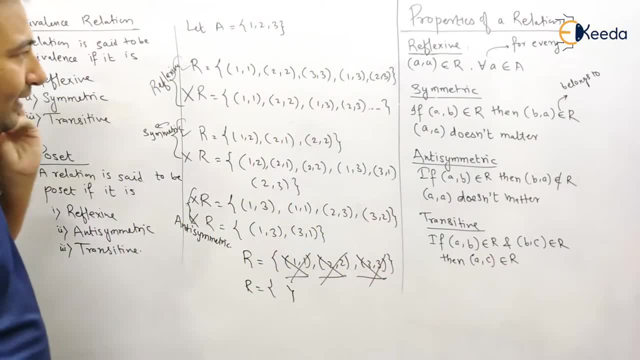 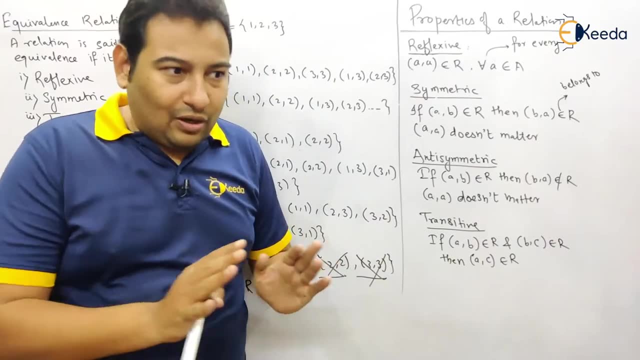 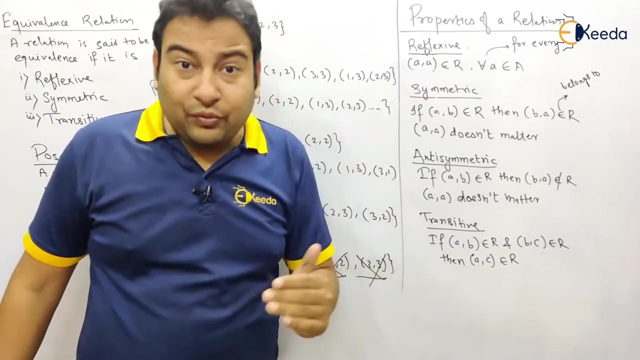 so what you're going to do, see, uh, i don't have space here to write, so whatever the discussion that we did, so first you watch this video without writing down anything. there is one more transit is left, so that we're going to cover, so don't worry. so what i'm saying is: first you watch this. 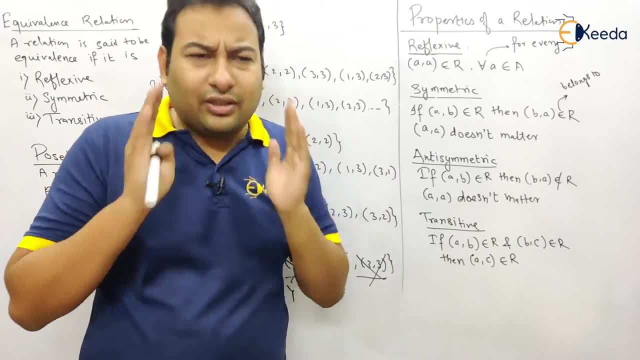 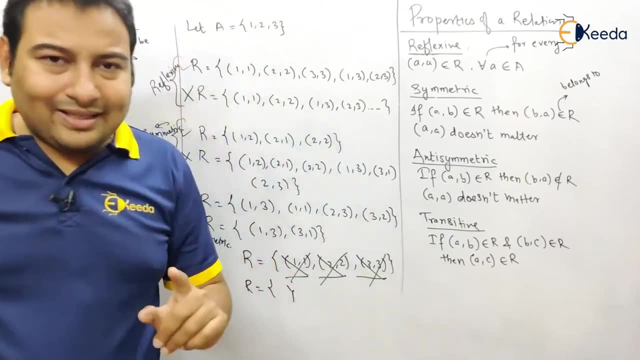 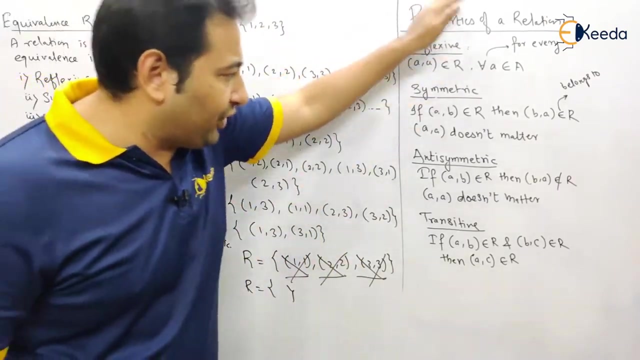 video, the entire video, without writing down anything, just watch, just watch with the full concentration, everything, keep aside and just concentrate, full concentrate, and watch this video once and then for second time when you're watching. try to copy all these things. first of all, you need to copy the properties and the example. this is your reflex, you example this. 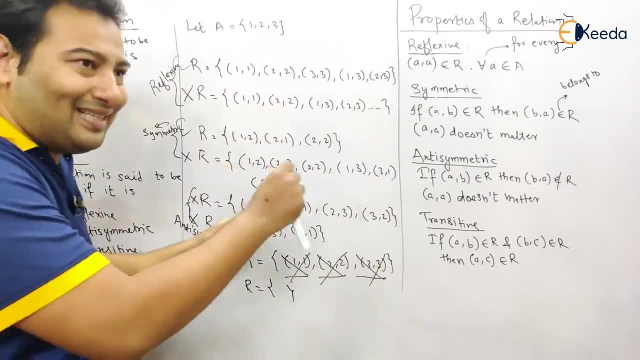 is not reflects you. this is symmetric, this is not symmetric, and so on. whether it is anti-referential or not, this is not symmetric, and so on. whether it is anti-referential or not is symmetric, so that you need to copy examples. you need to copy, so you need to pause the videos. 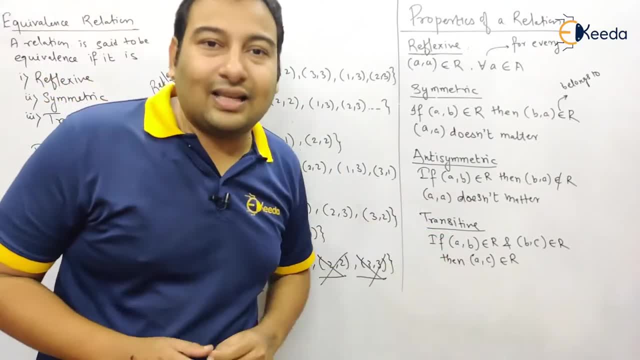 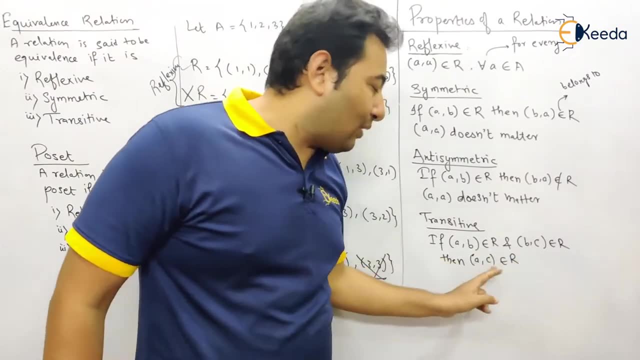 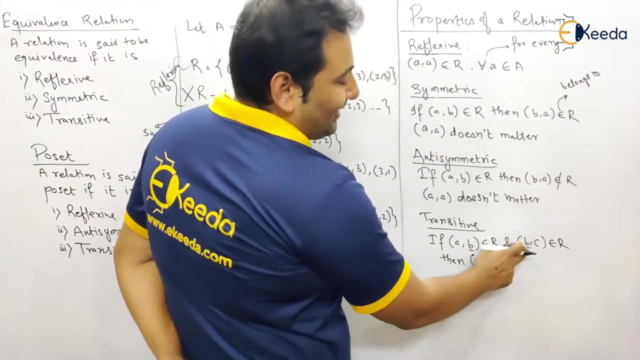 again and again and you need to copy. so let's move on and let's discuss the last. that is transitive. so transit is very simple. if a comma b belongs to r, b comma c belongs to r, then a comma c belongs to r. that means c. it is ending with b. it is starting with b, a comma b, b comma c, then a comma c. so what? 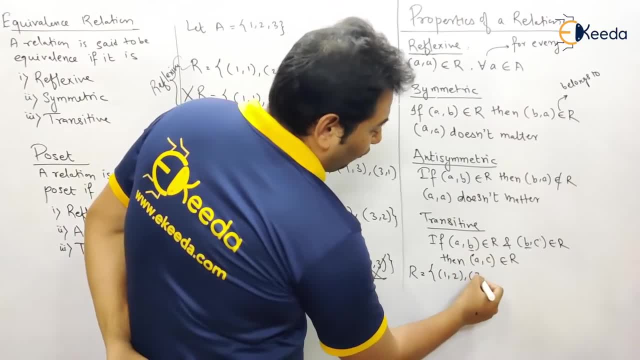 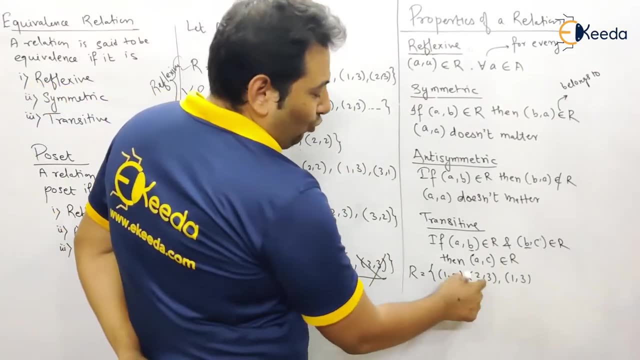 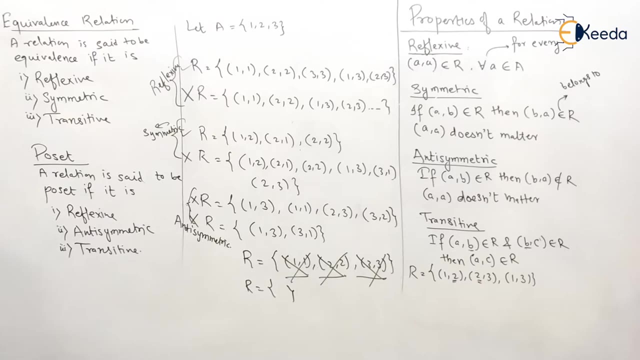 do you mean by that? let's say you have one comma, two comma three, then one comma three. see here: 1 comma 2, 2 comma 3, then 1 comma 3 must be present. if this is the case, then it is a transitive statement. so transitive statement. you need to check, suppose. 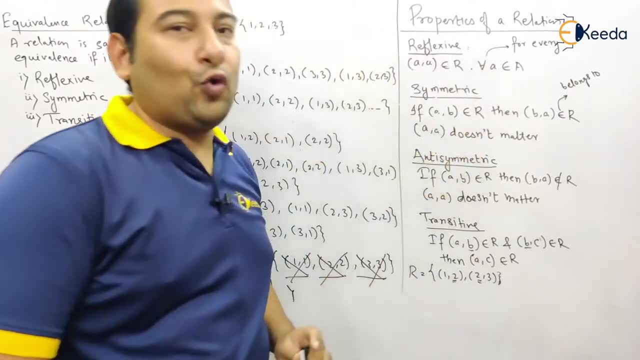 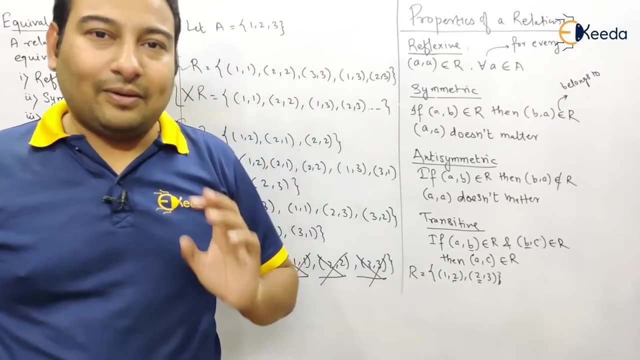 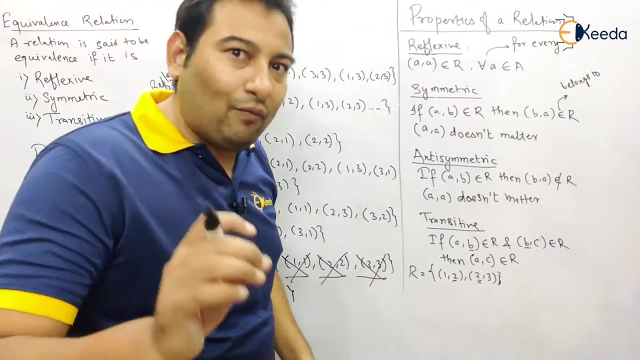 suppose you have only this, then is it transitive? no, it's not transitive. why? because one comma two, two comma threes, then one comma three must be present. then it's not a transitive statement. last point, very important point: full concentration on board. very last point: suppose you have only one. 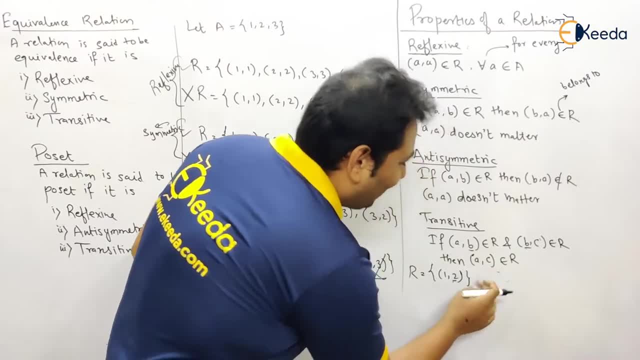 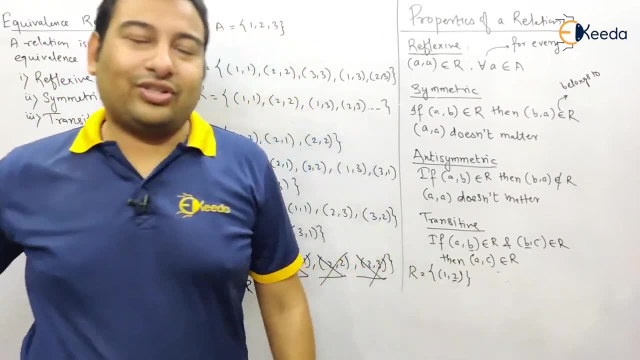 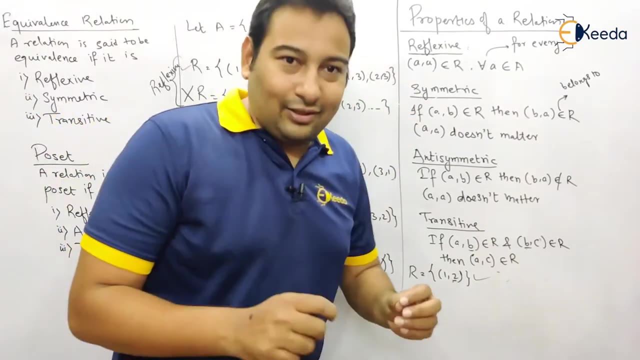 element now. please tell me whether it's a transitive statement or not. only last point element, that is one comma two. please tell me whether it's a transitive statement or not. yes, it's transitive, why? see again, you need to understand the english language, basic language, see. 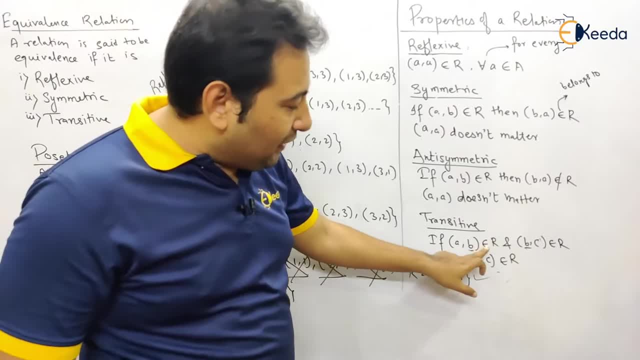 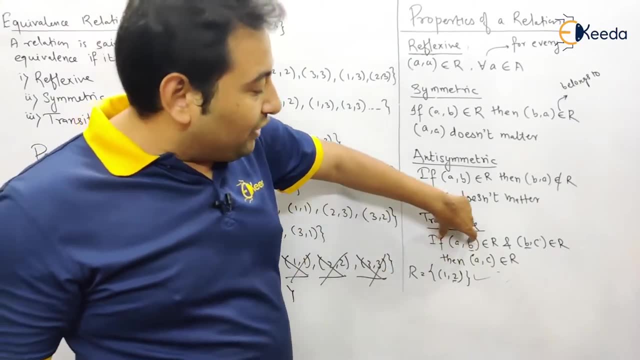 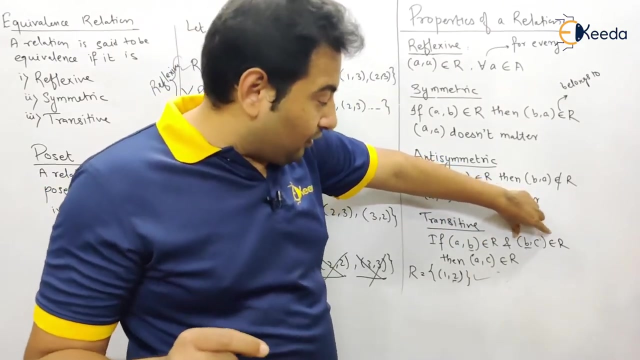 what do you mean? see read the statement. if a comma b present and b comma c present, then we're going to check for this. that means these two condition must be present: a comma b and b comma c. these two condition must be present, then we can check for this. 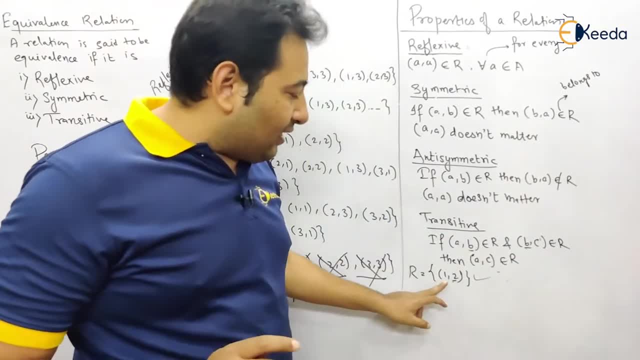 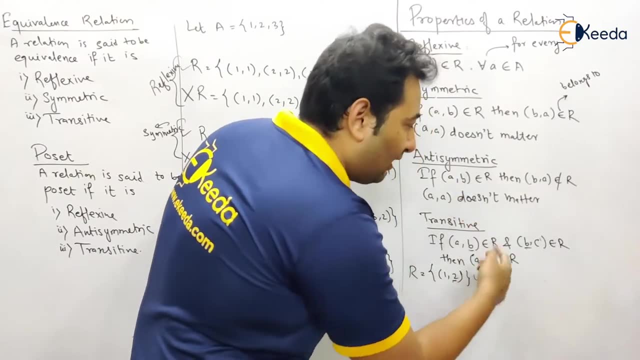 here. in this case a comma b is present and for second condition to be fulfilled, there should be a comma b and b comma c present. then we can check, for this should be a term that is starting from b. that means there has to be a term which is starting. 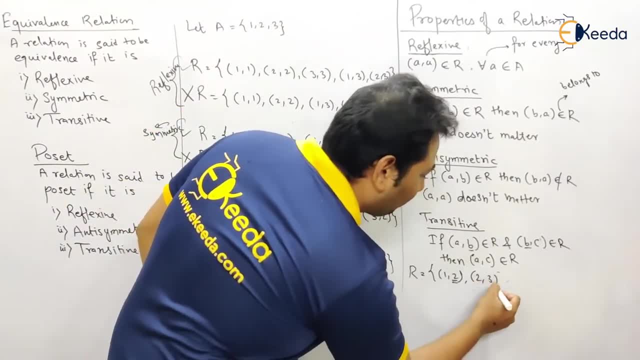 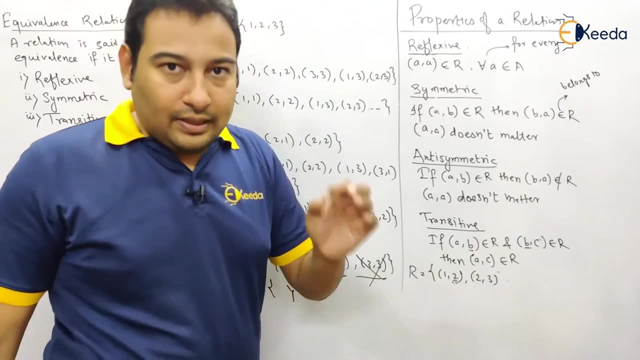 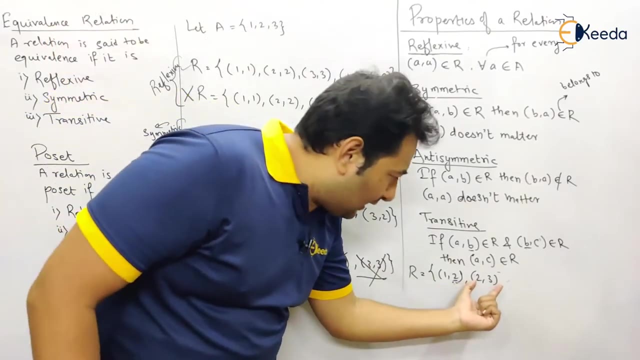 from b, b, b. here is two, so there has to be some term which is starting from two, so that you can check whether the third term is present or not. what i'm saying? a comma b, b comma c. there has to be an element which is starting from the b. if it is not present, 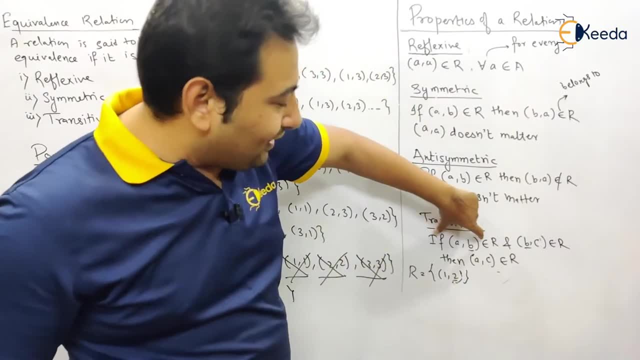 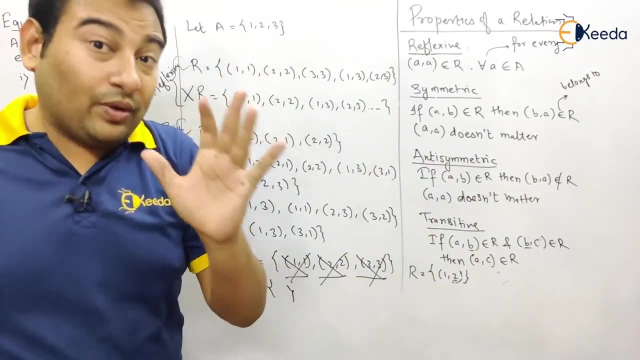 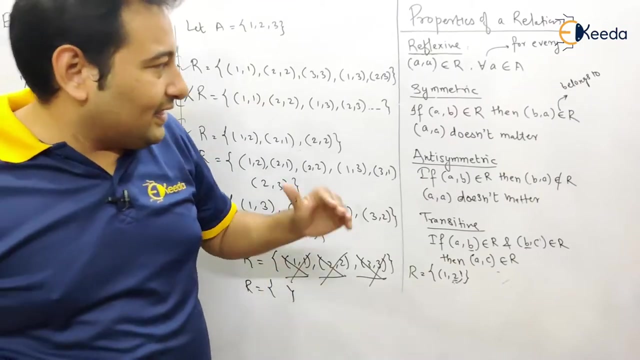 if it is not present, is not present, that means only this condition is present. this condition is not there, then it is by default transitive. this point is very important: only one term is present and the second condition is not present, then it is by default transitive. the same story we discussed. 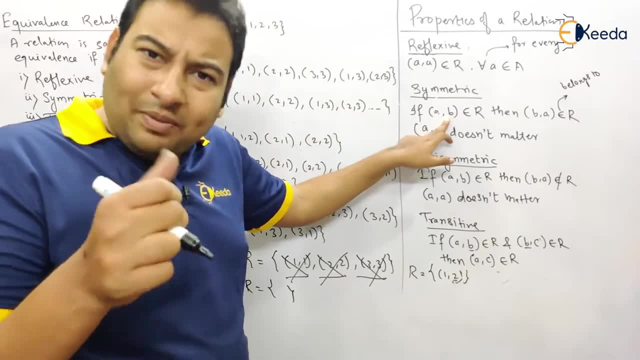 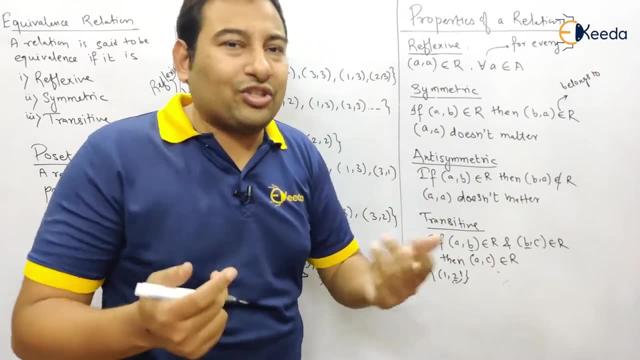 in symmetric and стор um. what i discuss is symmetry. if a comma b is not present, if it is not there, it is by default symmetric. no need to check this. if it is not there, how to check? how you can check? not possible. the same story is here. 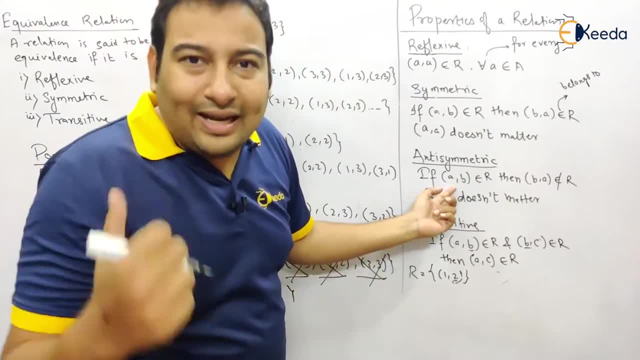 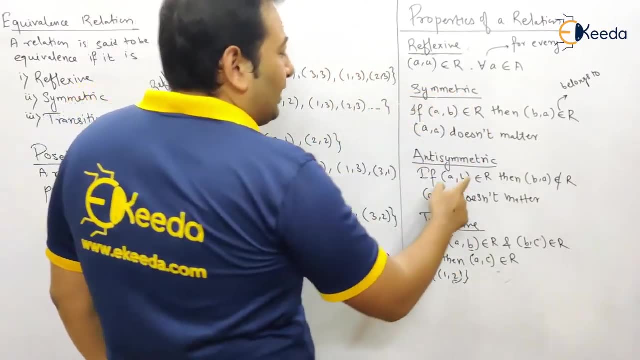 if a comma b is not present, it is by default anti-symmetric. that means, see, here there is only one condition. if that condition is not present, it is by default symmetric. if the condition is not present, it is by default anti-symmetric function to be transitive or 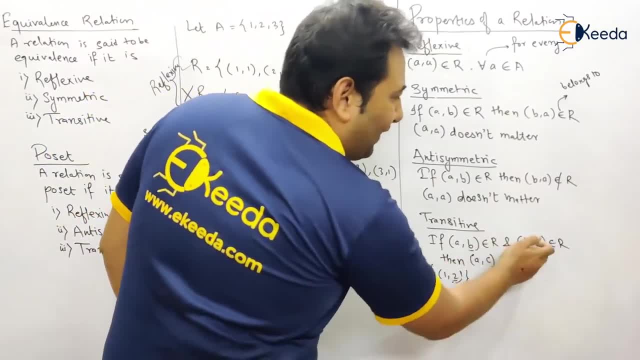 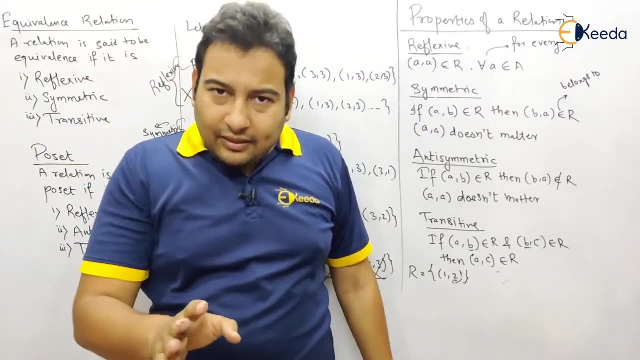 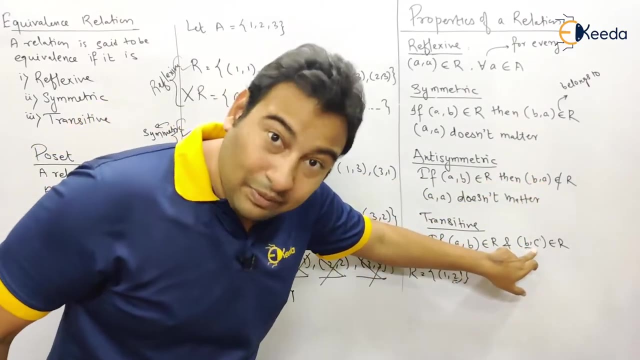 say a relation, to be transitive, both the condition must be present. if they are not present, it is by default transitive. so summary is: if the condition is present, well and good. then you check. condition is present, then you check. condition is present, then you check conditions present, then you check if condition is not present. a comma b is not there, it is by. 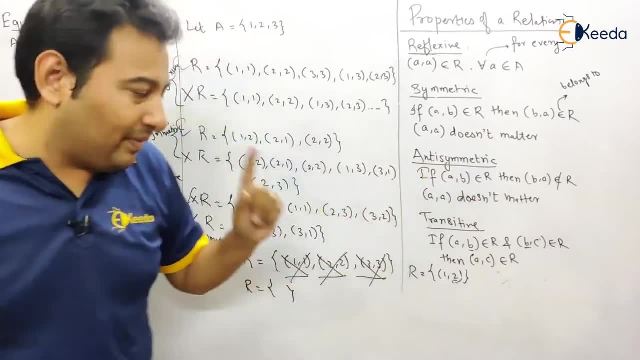 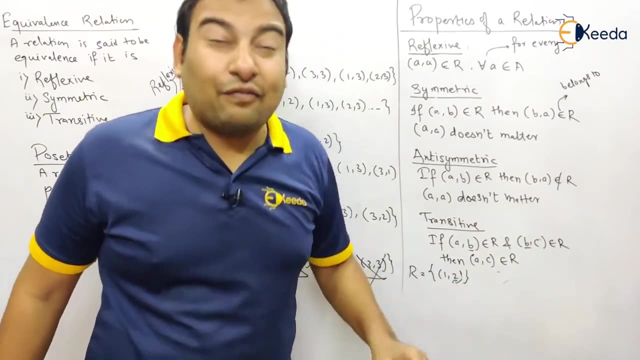 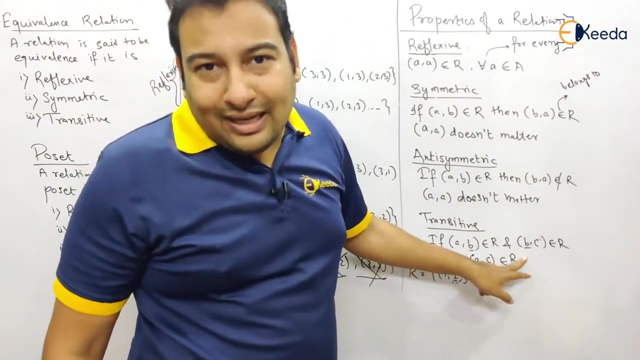 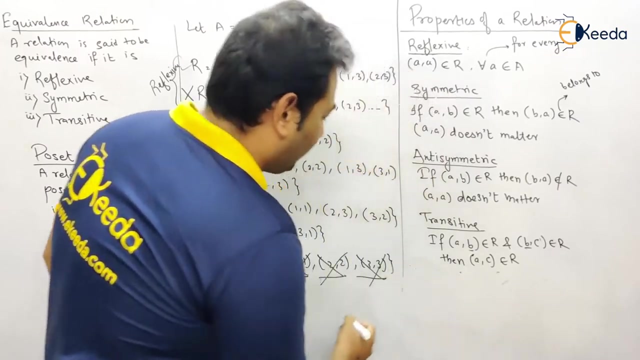 default symmetric. a comma b: not there. it is by default anti-symmetric- see here. if both the conditions are not present, it is by default transitive. see here: 1 comma 2. only one condition present. second condition is not there. it is transitive. 1 comma 2. let's say empty set. let's say empty set. please tell me this: empty set satisfies. 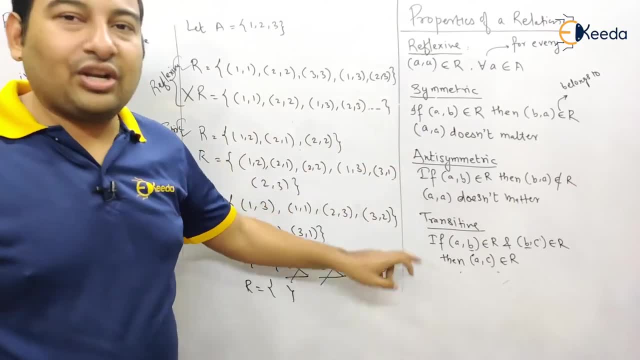 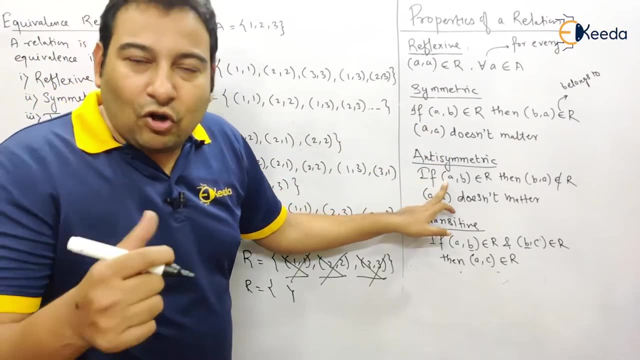 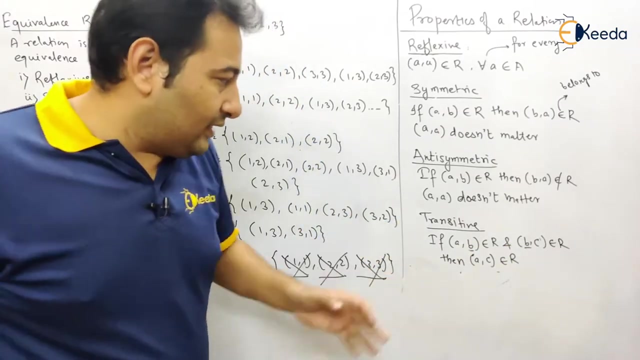 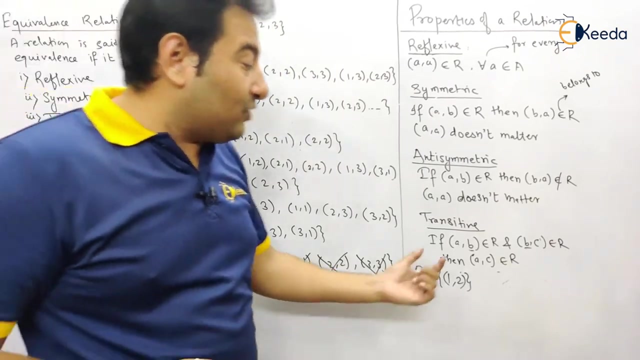 how many properties? symmetric, anti-symmetric, transitive. all why? because there is nothing to check. a comma b not present by default- symmetric. a comma b not present by default- anti-symmetric. both the conditions are not present by default transitive. are you clear with this? and if you have only 1 comma 2, then what? if you have only 1 comma 2, that means only. 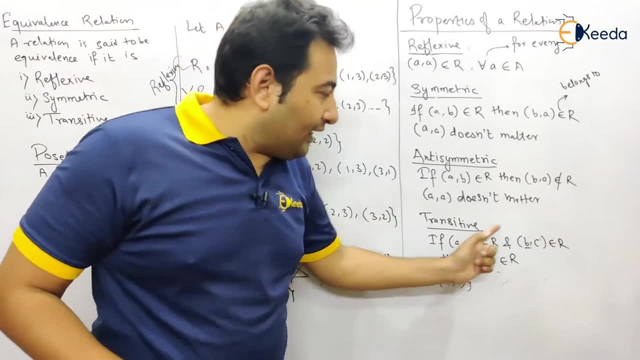 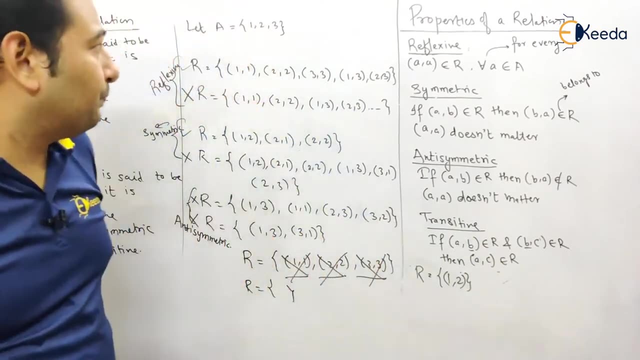 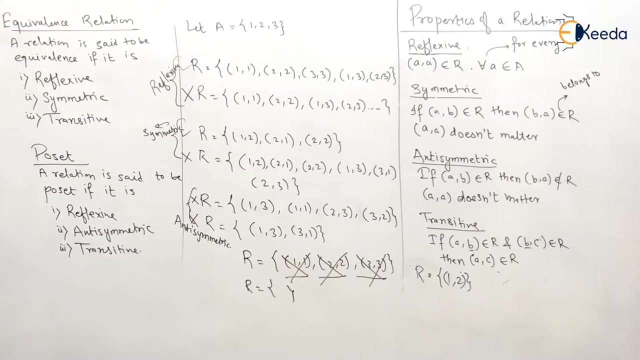 one condition, second, is not present by default. transitive. both the condition must be. chair must be present. so that will check the third condition to be true or false. are you clear with this? this is one of the most interesting topic that i like to teach and i enjoy and 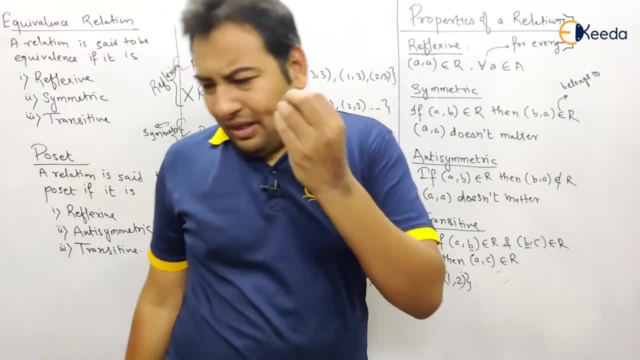 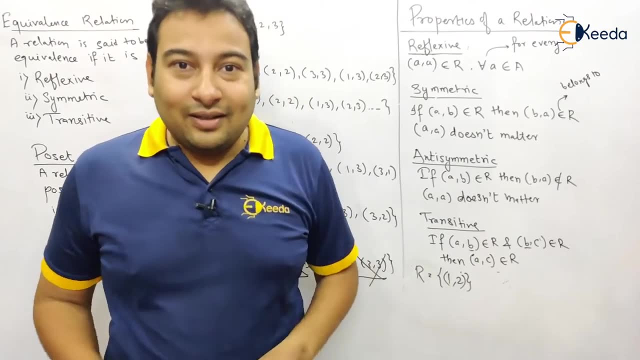 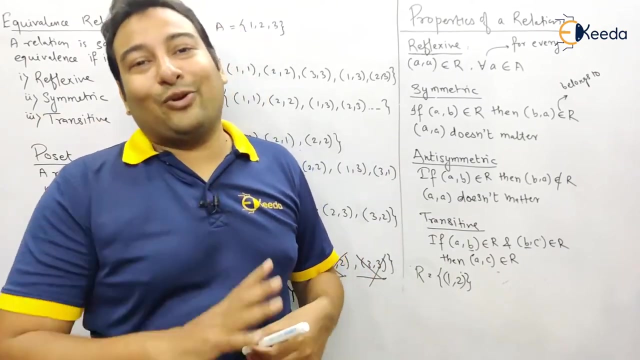 students even enjoy. but see, to be very frank, if you're watching this video for the first time, you will not understand. if you understanding well and good, but most of the students will not understand while watching this video once, so at least you need to watch twice or thrice. 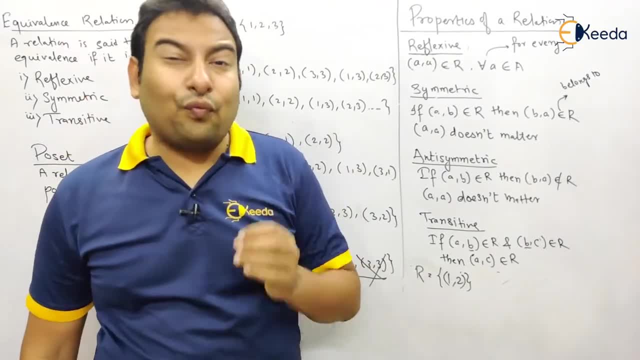 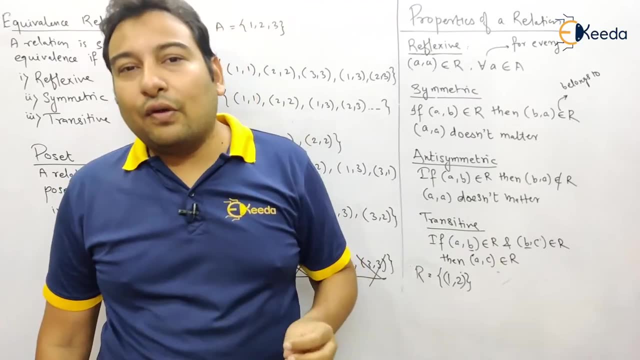 so that the concept will be clear to you and let me tell you, friends. so very important video. it's very important video. further topics are dependent on that, so you cannot skip, and some of my favorite questions are on gate and mcq. so what are we going to do? 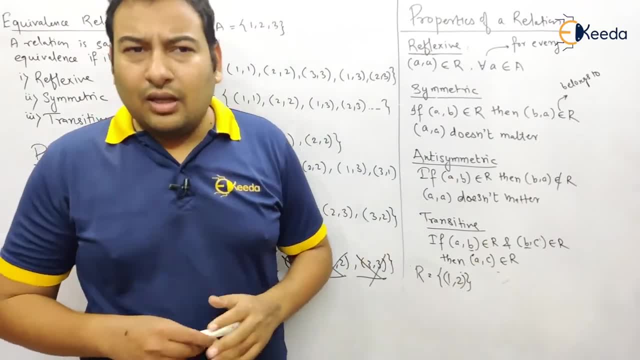 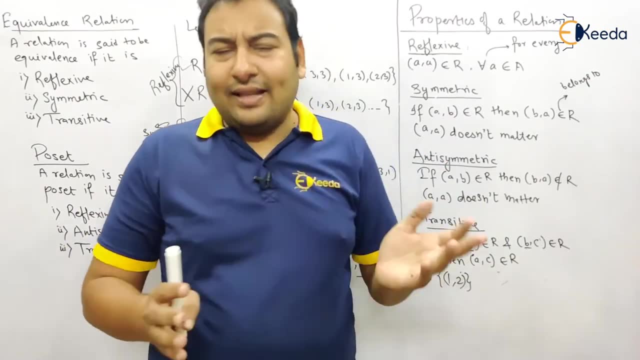 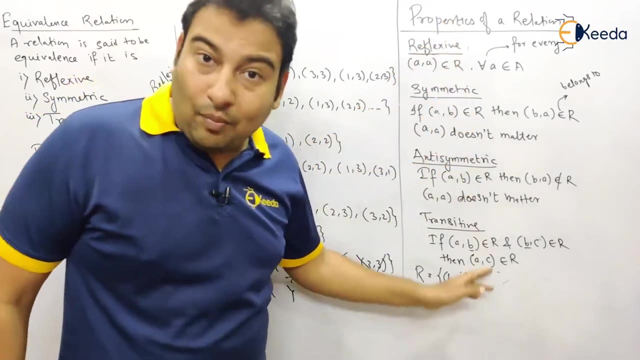 first time, watch the entire video without, um, without writing down anything, just full concentrate and, uh, you will understand few things. obviously i think uh, uh, you'll not, uh, you'll not get the full video. then this: while watching the video second time, write it on the properties properly. 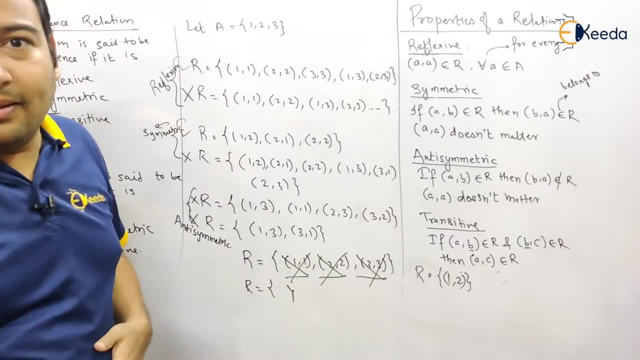 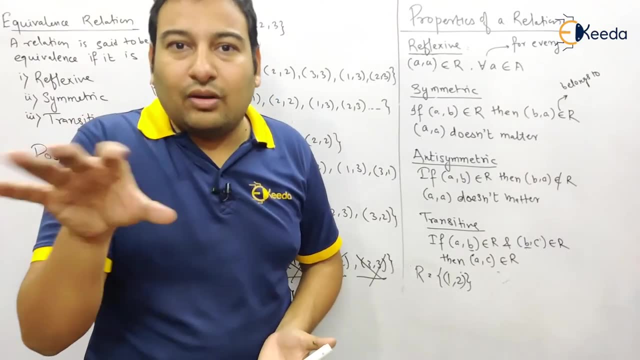 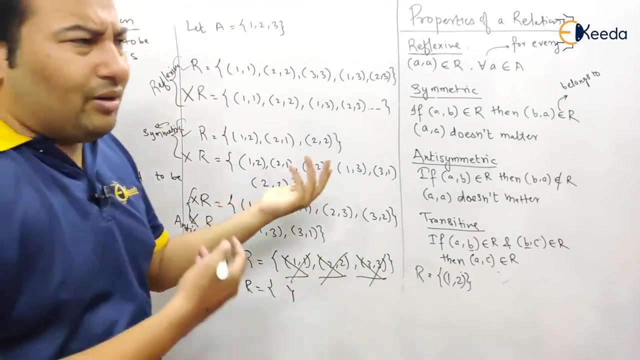 and the example that we discussed, all the examples that we discussed. pause the videos and write it down, all the examples, and in bracket write it down: uh, different property. that is satisfying. this is reflexio. this is not reflexio. this is symmetric. not symmetric or a relation, maybe not. 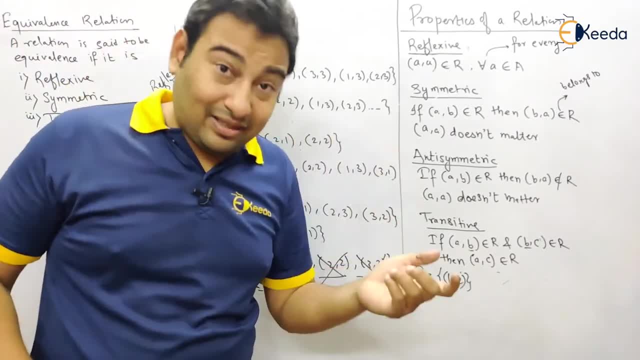 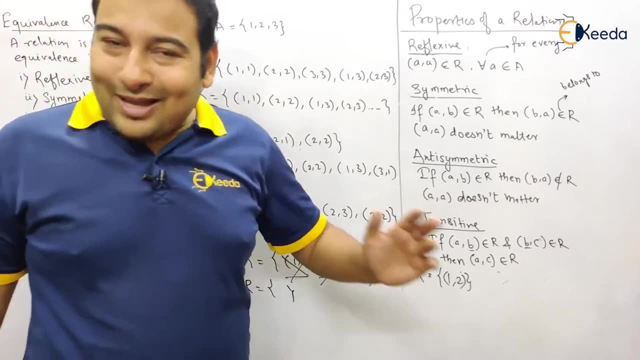 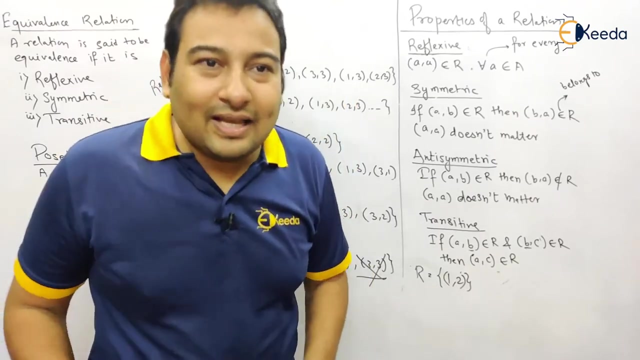 symmetric as well as not anti-symmetric, and which are the relation with a symmetric and symmetric, both and so on. so that's it for this video. after watching twice thrice, still, you have a confusion. so don't worry. in the next video we'll be discussing 10 examples in which we'll be with. 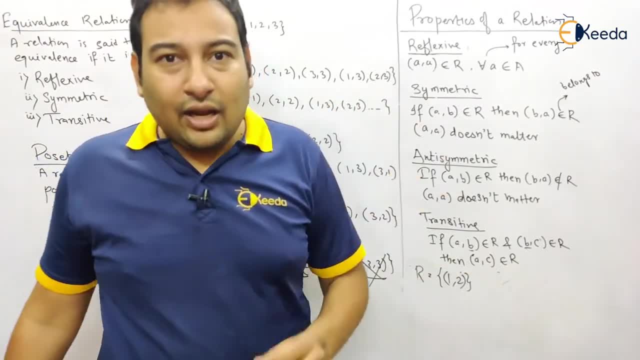 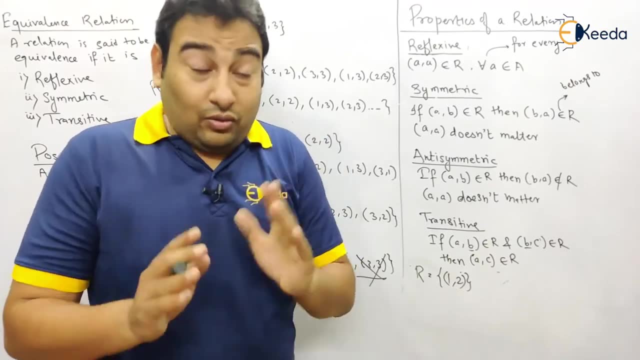 the action. the relation will be aswatch, which is not epa like our way, because animated, depth based help of 10 examples. we'll discuss the properties again. so if you're not understanding after watching two, three times, don't worry. skip this video and come. don't skip once you're done with this. 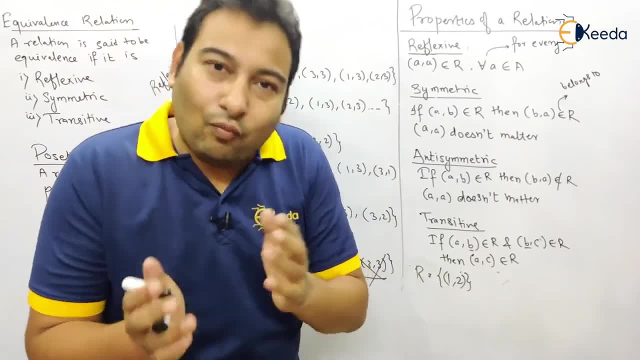 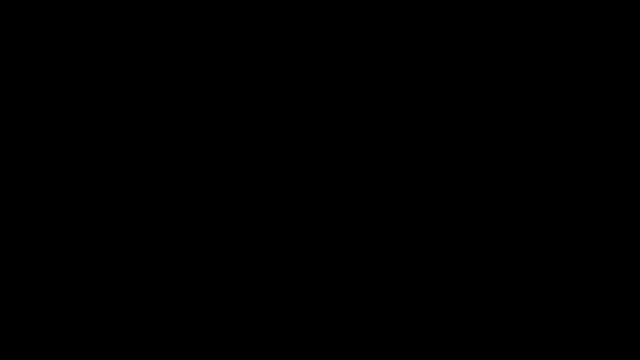 if you're still not understanding, don't worry, go watch the next video. the topic will be very clear to you. hope you understood. thank you you.